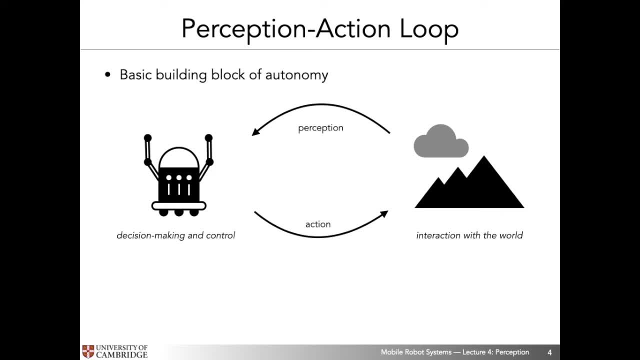 role is. So, again, to recall what perception is, perception algorithms infer information about the state of the world, And they do this in such a way that the robot can use their output to make decisions about the actions that the robot would next take. And since we're focusing on mobile ground robots, 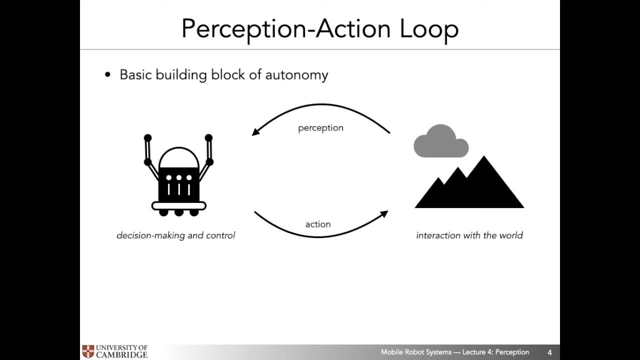 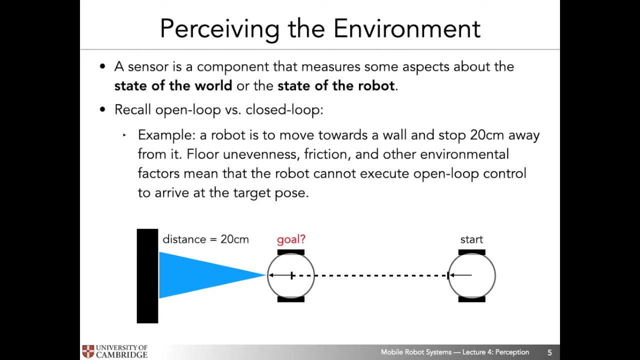 in this course. perception, in our case, will really be related to localization and navigation, And the decisions that will then be based on these outputs from the perception modules will be related to motion and navigation. So how do robots perceive the environment And how do sensors actually lend themselves to this problem? 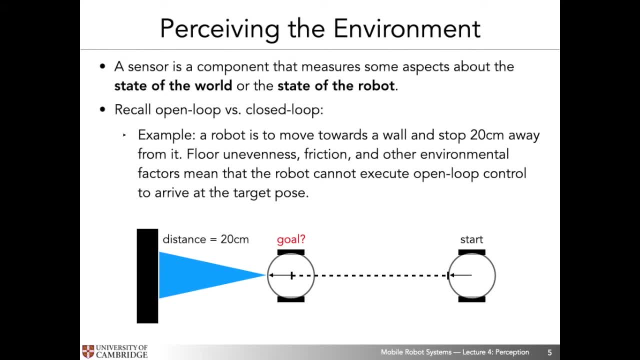 So, first of all, what is a sensor? Maybe we can start by defining what a sensor actually does for us. So a sensor is a component that measures some aspects about the state of the world or the state of the robot. So when I talk about the state of the world, for example, this could be: 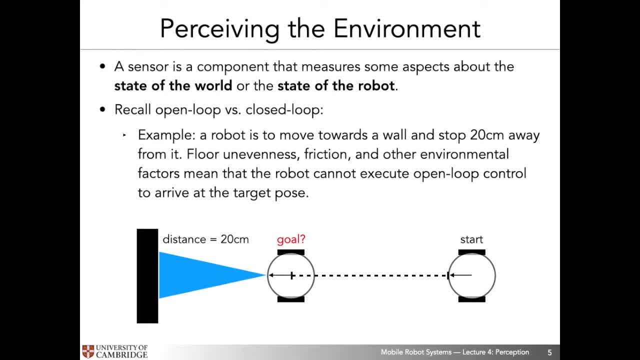 measuring the position of a given object, that is, not the robot itself. And when I say state of the robot, for example, I could be trying to measure the position of the robot itself in some coordinate frame, a global coordinate frame, for example. But the state can also be something that is not related to geodesics, For 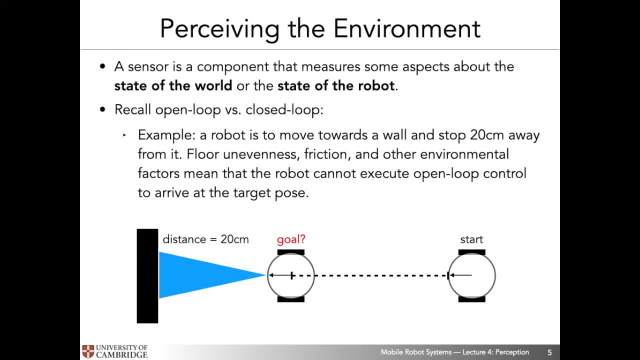 example, a robot could be trying to infer the intention of another agent, right? So this could be some sort of state of the world that the robot is trying to estimate. To give you a very concrete example, if you think about autonomous vehicles- one of the things that they would ideally be able- 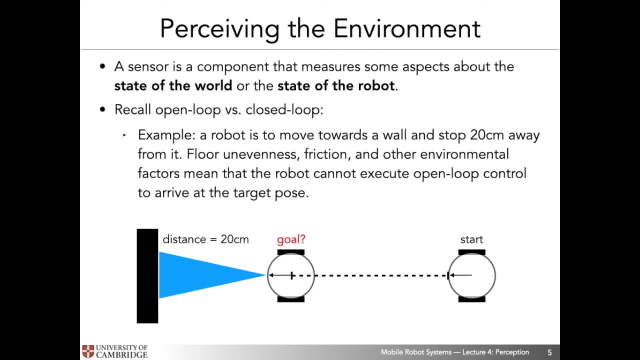 to do is to infer the intention of, say, pedestrians or other vehicles around them, Because if they can infer those intentions, they could plan out their trajectories as a function of the trajectories of the autonomous agents around them, right? So this is a kind of a state of the world that robots might 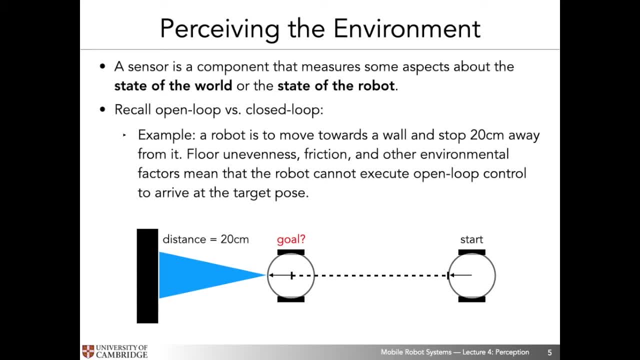 want to be trying to estimate via perception algorithms. Now, I'm just going to make a very simple example in the context of open versus closed loop control, which are concepts that you are now very familiar with, right? So what we would like to do here in 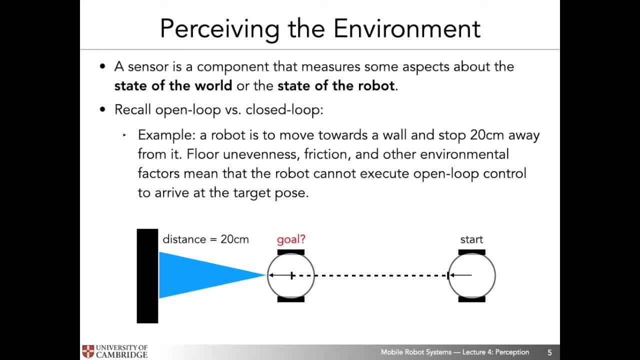 this little, very simple example is we want a robot to move towards a wall and stop at a distance of 20 centimeters to that wall. Now, if we think of closed loop control, you'll recall I always mentioned what we have: this oracle that is telling the robot what its state is and allows it to. 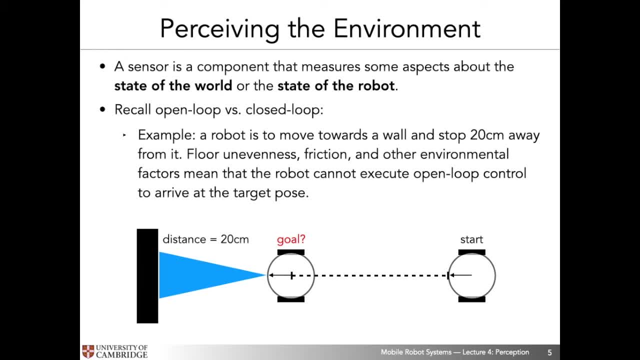 implement the closed loop control paradigm right. So if we think of closed loop control, we have a constantreating of 2 אנחנוs không в Sénergy đ 모습. So if we think of closed loop control, the magician moves towards the wall. In another example, 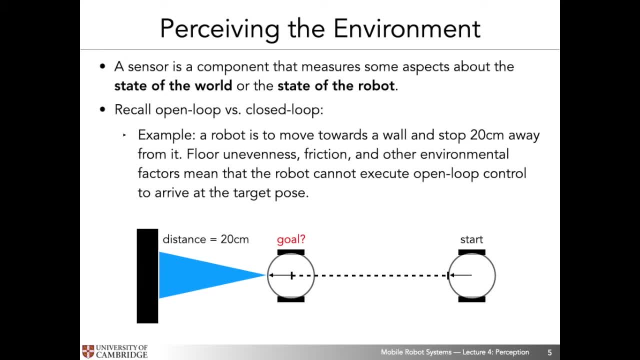 in this example, the robot could not move at a distance from the wall, So what we're meaning here specifically is that the robot is going to use the feedback on its distance to the wall to decide whether or not it's going to stop moving and what it needs in order to. 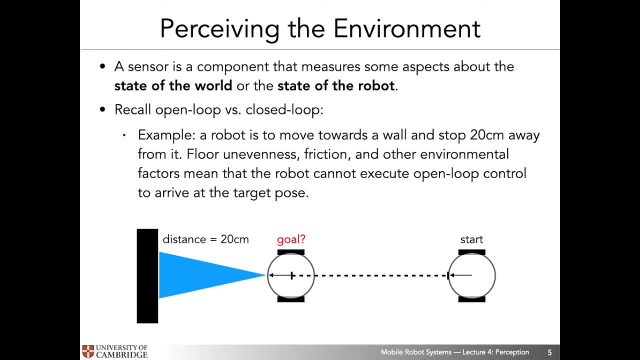 do this is simply some sensor and a perception algorithm that allows it to infer how far it is from that wall right, And so this is how sensing and perception connects to the idea of closed loop control, and you'll recall the alternative here is open loop control, where the robot maybe knows. 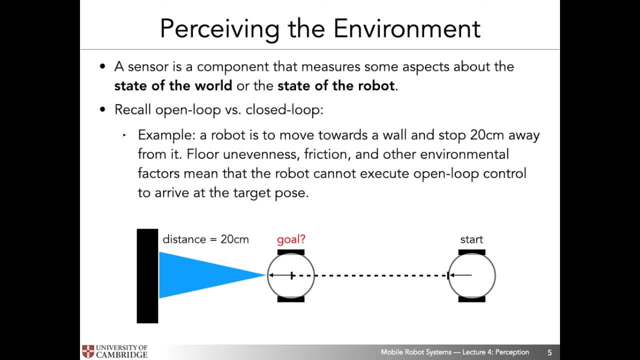 that the robot needs to be removed from that wall to know that, although it was not shut down, it was in the world of closed loop control, knows its starting position and it might be able to track how far it's moving, but it's not going. 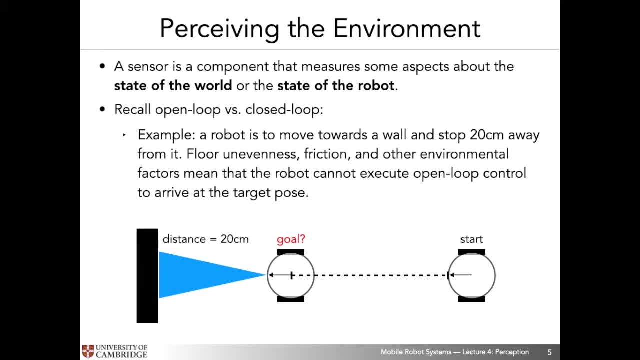 to be using any sensors or perception to actually tell it how far it truly is from the wall. so inevitably, in open loop control, the robot will stop at a distance from the wall that is probably less precise than the distance it would have stopped from the wall at had it been using 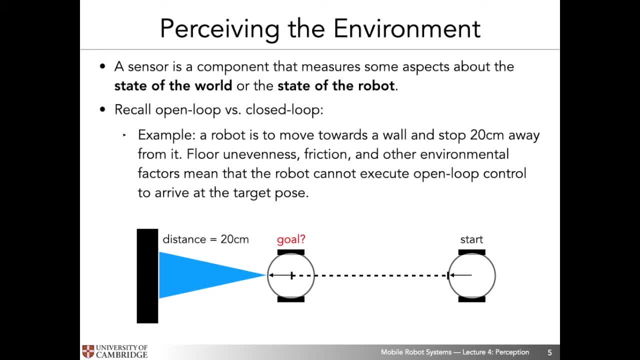 closed loop control with some extra receptive sensors that are telling it how far it truly is from the wall. okay, but obviously this is not always true what i just said, because it will depend on the sensors that you're using to measure those external aspects. right distance to wall. 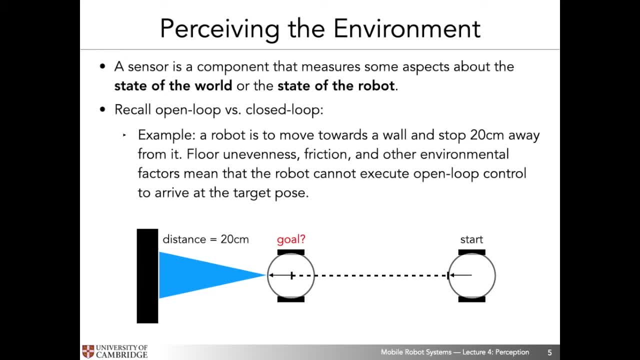 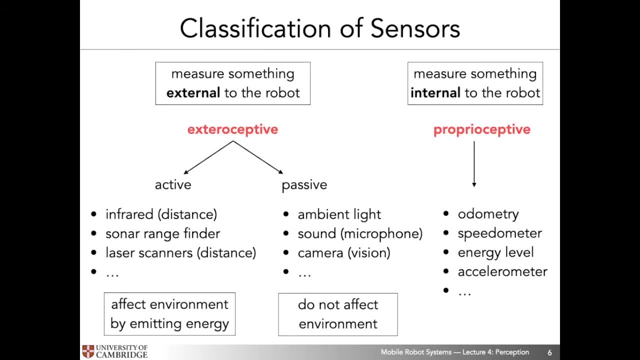 versus the precision and accuracy of the sensors that the robot is using to measure its own movement. right, so of course we have to take that into account, but this is just an example that brings perception and sensing into the context of open loop versus closed loop control. so now, in terms of sensor types, at the 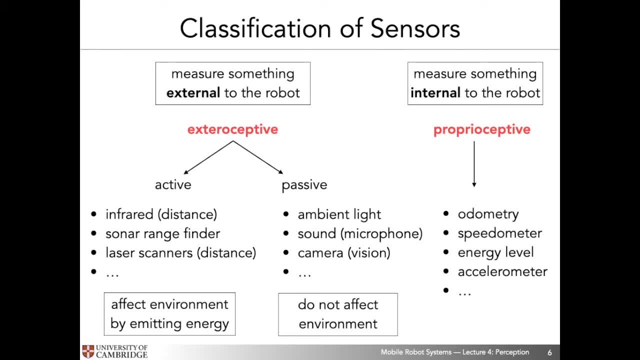 very highest level. there are two types of sensors, right, so there are extra receptive sensors that measure something external to the robot and there are proprioceptive sensors that measure something internal to the robot. okay, so if we look at the class of extra receptive sensors, again, there are two types that we like to use to distinguish these. these sensors within this class. 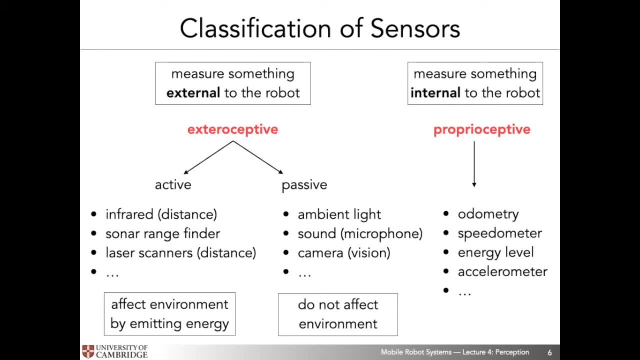 active extra receptive sensors versus passive extra receptive sensors. so the active ones are defined by the fact that they affect the environment by emitting energy. so, for example, we can think of infrared distance sensors that actually emit infrared light, right, and they then measure the received light intensity to determine how far they are from the objects that actually 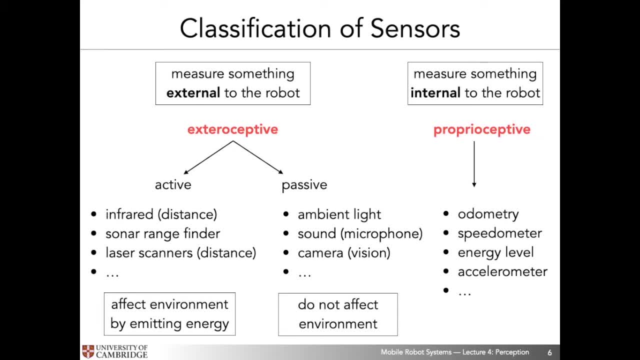 reflected this emitted light or emitted energy, right. we can also think of ultrasound sensors, which emit sound waves and measure the round trip time of flight. or we can think of laser scanners, right, that emit focused light. and there are many other examples of active sensors, but these are three of the most. 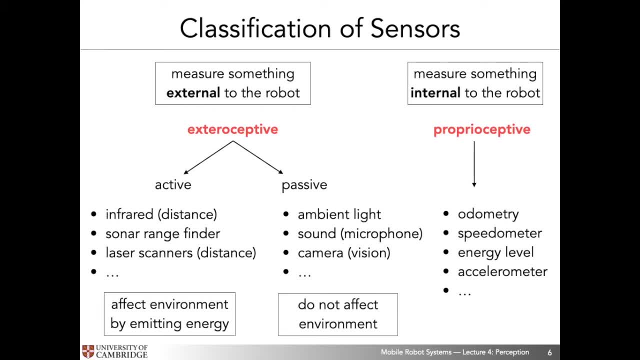 common or popular active sensors that are used in localization and navigation. in the class of passive sensors we have, for example, ambient light sensors. so these are the most common active sensors that are used in localization and navigation. so those could, for example, be infrared receivers, but those that do not actually emit any energy. 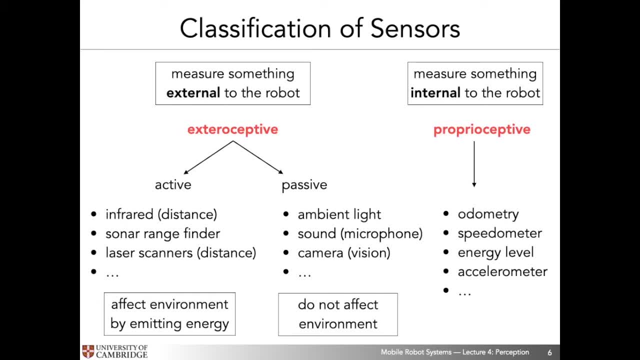 or we could be measuring sound, or we could be measuring- uh well, we could be measuring vision or camera. right, using a camera, i'm trying to estimate, um, the the visual state of our environment, without actually affecting it. okay, so the key thing here with passive sensors is: 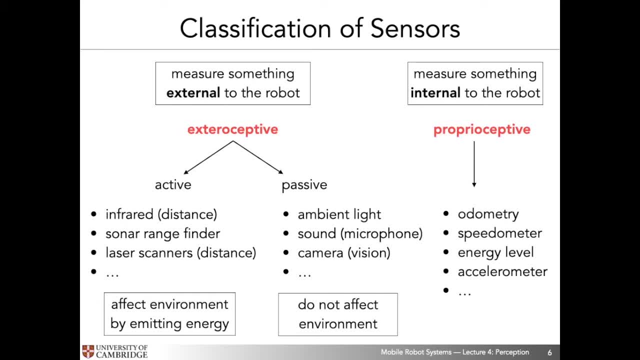 that they only measure incident energy and, of course, in various forms. right, so the different types of sensors are measuring different energy modalities. in the class of proprioceptive sensors, we have different types of sensors that measure something about the robot itself, and this is, of course, very useful not only in terms of navigation and localization, but also 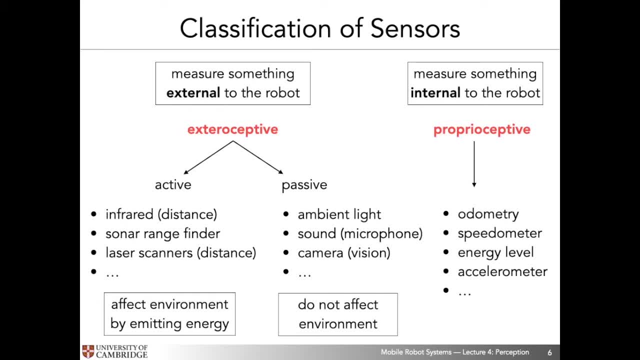 in order to manage the internal health of a robot. so i'm talking about, for example, energy levels or not the robot is off balance, right? if we're talking about walking robots and robots that need to maintain stability, so those kinds of sensors are also very important and allow the robots 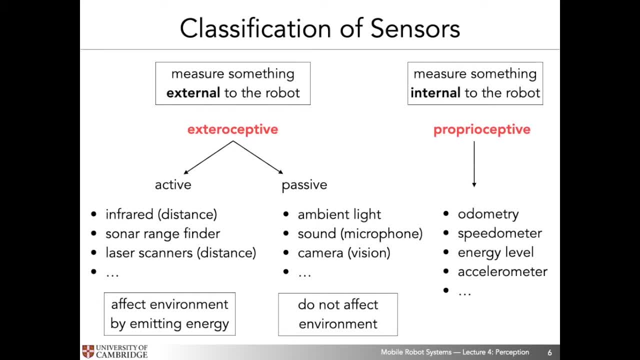 to achieve their tasks successfully and, as i mentioned in the previous slides, odometry will be a sensor or sensing foundation that we will talk about quite a bit in this course, because it's really important and crucial to one of the aspects that we'll be looking at that enable 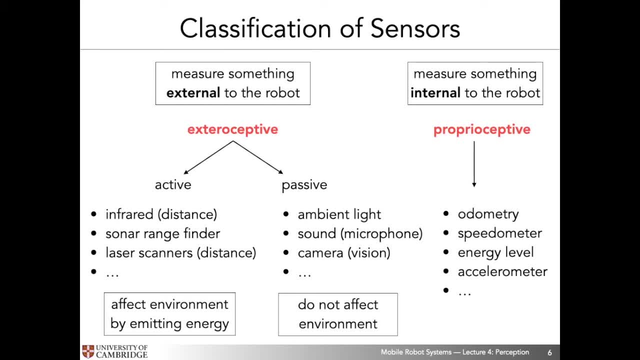 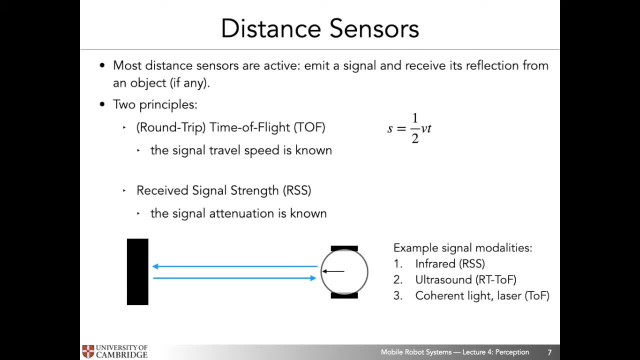 a robot to know where it is and where it is going. okay, so now let's dive in and look at a specific case study, which here is the class of distance sensors. so distance sensors are actually one of the most common types of sensors used for localization and 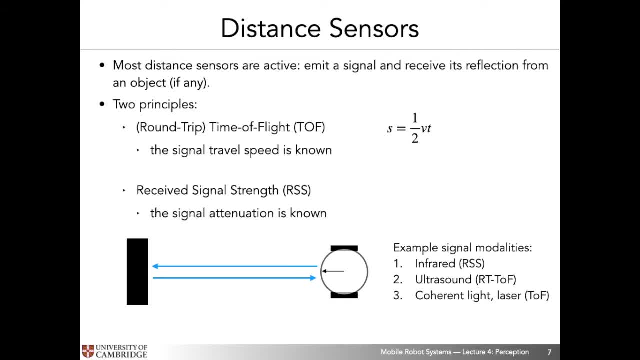 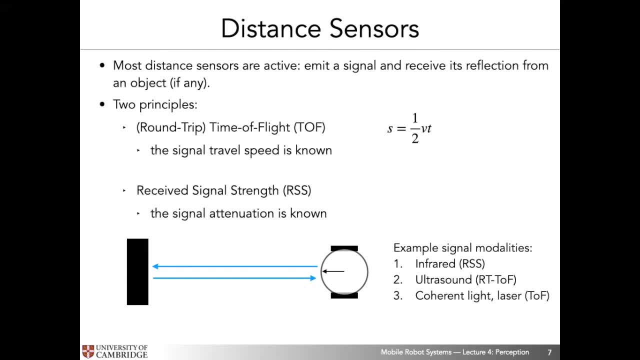 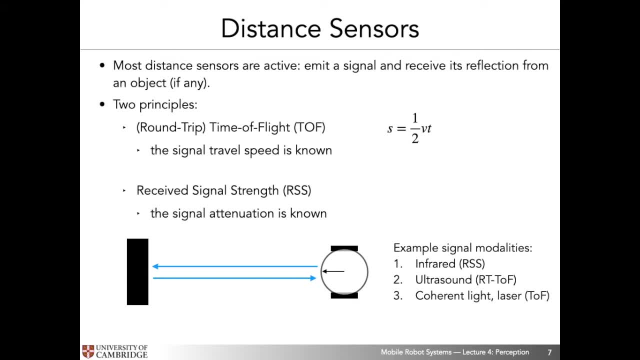 time of flight, where we make one assumption, which is that the signal travel speed is known, and once we know that quantity, we can then measure the speed of the signal travel speed, and then we can- and we can measure emission and receivable times of the signal. then we can infer something about. 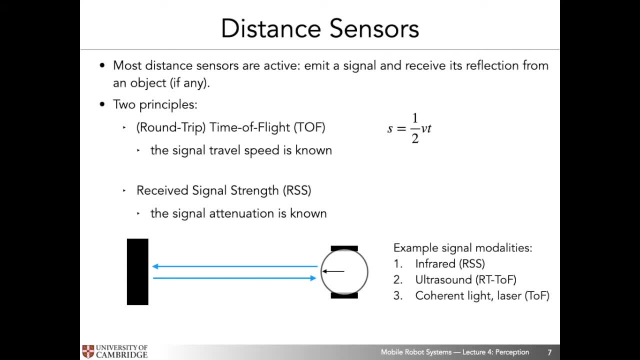 the distance between the robot body and any reflecting object. right, and this is how distance sensors relying on time of flight are useful. Then the second principle is received signal strength, where we make the assumption that the signal attenuation is known, right. so, in other words, we assume something about the model of the decrease in signal intensity as a signal propagates. 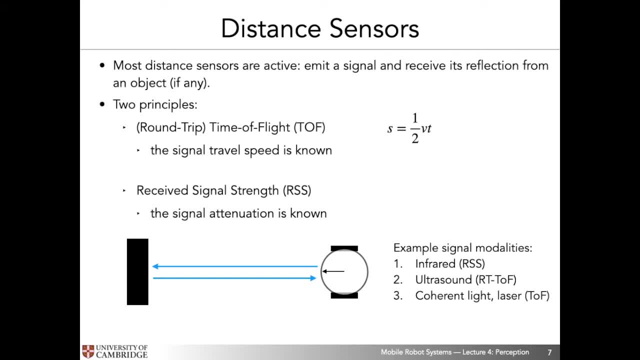 throughout space. so you know how signal attenuates over distance. Typically this is harder and more imprecise than round trip time of flight or time of flight, especially since signal attenuation is quite dependent on the environment and the environment is generally unknown, because that's what we're trying to perceive, right. 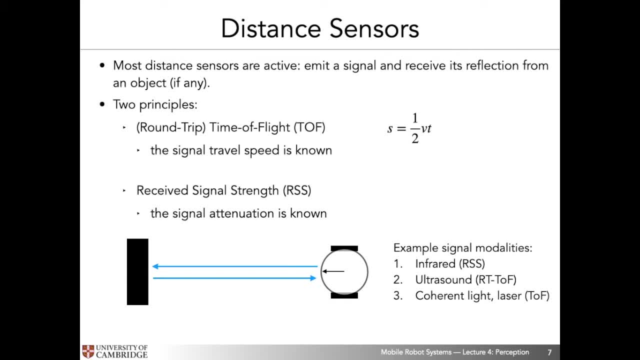 But these two classes are the more popular and well-known sensing principles and, for completeness, we will be discussing examples that belong to both of these classes. So fitting or matching up examples of actual sensor modalities to these measurement principles is one of the things we're 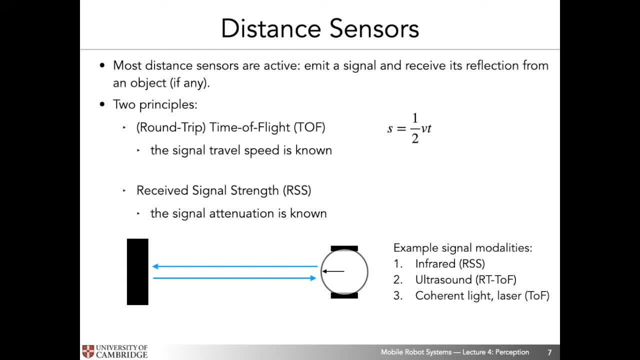 going to do in this lecture. So we are going to look at infrared sensors that rely on received signal strength. We're going to be looking at ultrasound sensors that rely on round trip time of flight, and we're also going to look at infrared sensors that rely on received signal strength. 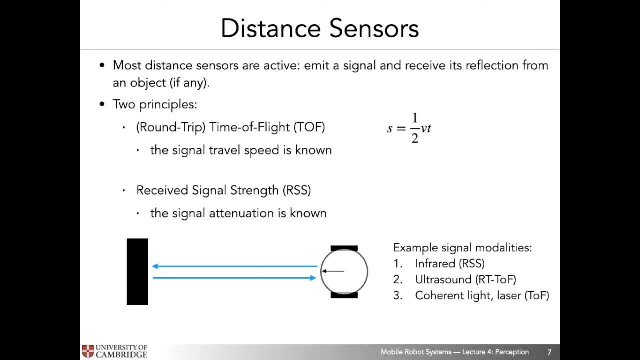 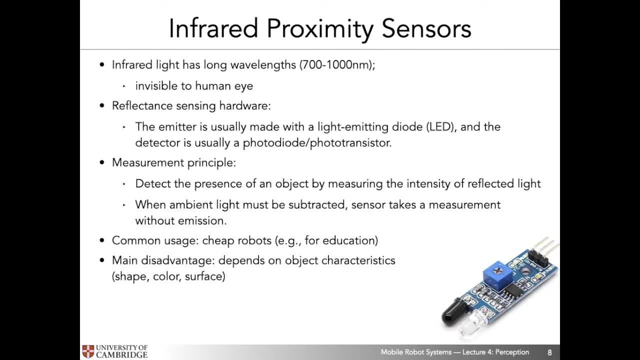 So we're going to be having a quick look at how laser sensing works, also based on the time of flight measurement principle. So let's take a look at our first example, which is given to us by infrared proximity sensors. So infrared sensors, or infrared proximity sensors, as their name already gives. 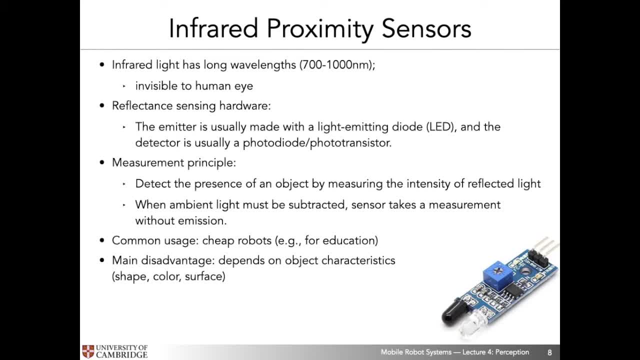 away. they rely on infrared light as their main sensing modality and this is useful because infrared light has long wavelengths invisible to the human eye and they can sense the light and can still be relatively easily sensed by relatively cheap sensing hardware. So in the particular case of IR sensor, the emitter is made with an LED diode and the detector is usually a. 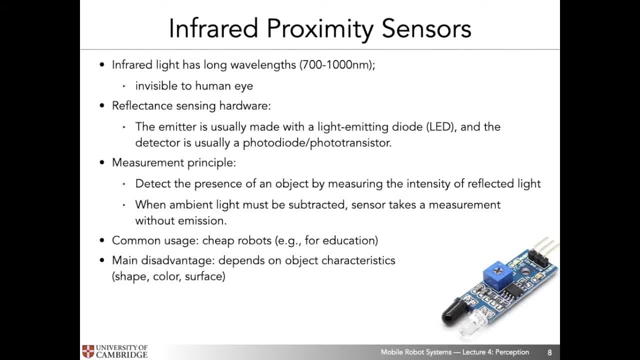 photodiode or a phototransistor. So the measurement principle is based on the fact that we can detect the presence of an object by measuring the intensity of reflected light. So recall that infrared proximity sensors are active sensors and we assume here that the light intensity decreases. 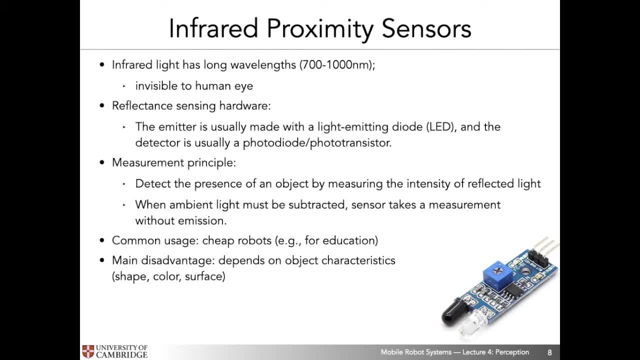 with the square of the distance from the source, and this relationship can be used to then measure the approximate distance to the object When ambient light must be subtracted. sensors can also take a measurement of the light without emissions, or we can alternatively also put a passive optical infrared filter in front of the detector to measure the light without emissions. 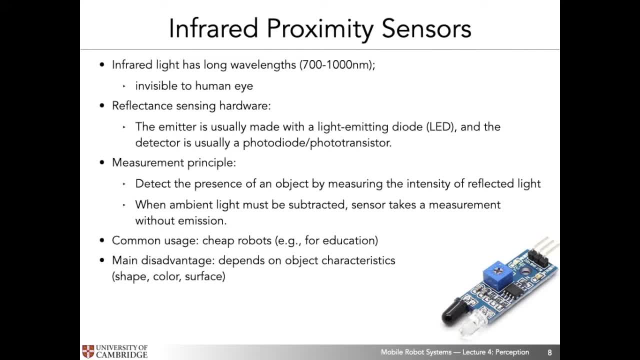 So those are various ways in which we can use infrared proximity sensors. As I mentioned before, they're very popular, especially for educational robots or cheaper robots, because infrared circuitry and the infrared sensors themselves, those photodiodes, are very cheap to produce. They're standard off-the-shelf components and the little PCB boards that we use for them are also very easy. 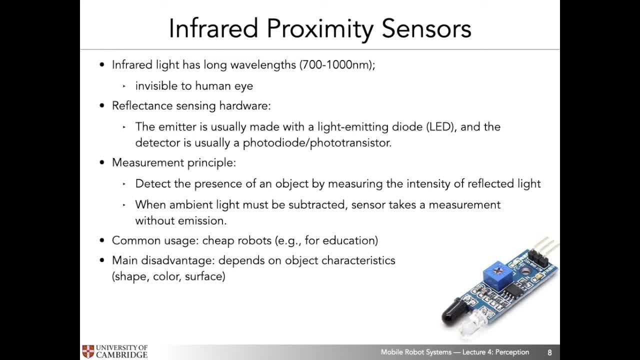 to construct and print. Now, the main reason why we use infrared sensors is because they're very powerful and they can be used in many different ways. The main disadvantage of infrared proximity sensors is that they actually so the signals, or the that are that are reflected, and how they're. 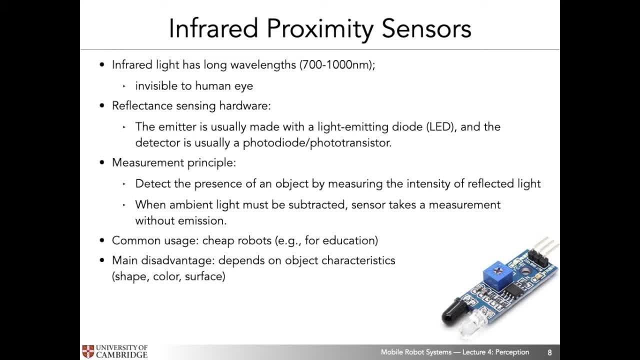 being reflected will strongly depend on the reflecting objects characteristics. So, for example, if the reflection happens on a smooth surface, the reflection will be much stronger than if it happens on a rugged, non-smooth surface, where we have light being scattered in various directions, versus with smooth surfaces, all the light being focused and coming back to the receiver. Similarly, you'll 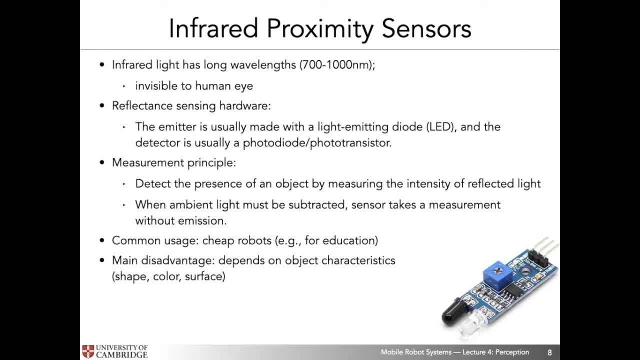 find that white surfaces tend to reflect more light and darker surfaces tend to absorb more light, and this will also affect the receiver's sensor measurements and will in turn affect the estimated distance to the given objects. So those are the main disadvantages of using infrared as a sensing modality for distance. 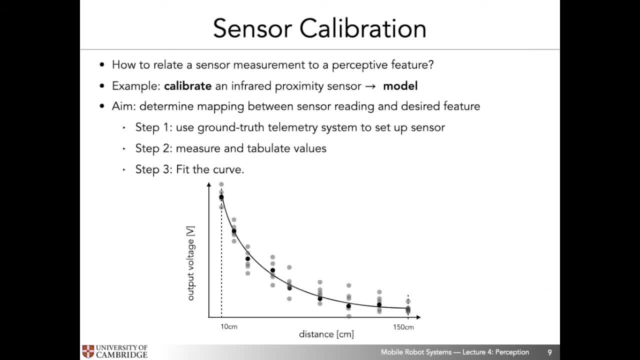 Now, the key question that we ask ourselves- and this is relevant to any type of sensor- is: how do we actually relate a sensor measurement to a perceptive feature? right, So a perceptive feature can be anything really, but it tends to be the, the quantity that we're interested in, or that. 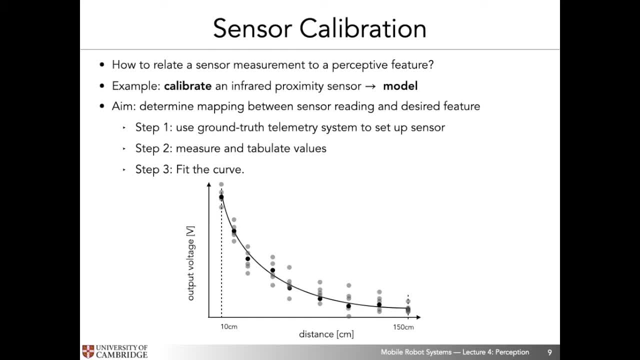 we can most usefully use within a perception algorithm, For example, distance. Distance is a perceptive feature and one way we can. You know we're not going to be using it like I used to and sometimes I can't do it. I should really increase the scale a little bit. I will not naturally increase. 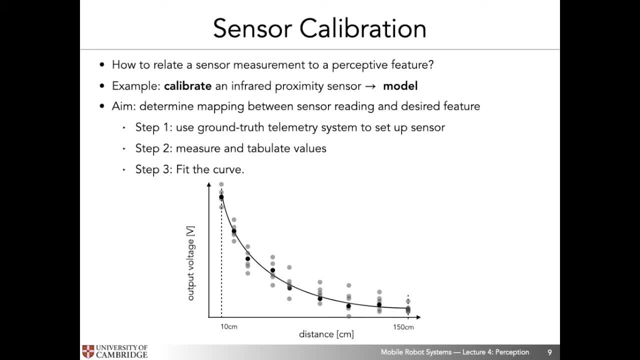 the scale, so it doesn't take it too long. So we'll use dedicate information and we can let this figure in until we draw some. create this relationship is through a process that is called calibration, And we're going to have a look at an example of how to calibrate an infrared proximity sensor. This process of 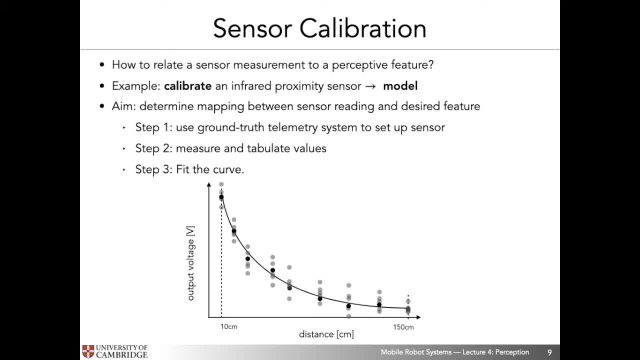 calibration. what it produces for us is actually a sensor model, And the sensor model is the formality that relates the output of a sensor to our perceptive feature. So the goal of any calibration procedure is to determine the mapping between the sensor reading and a desired 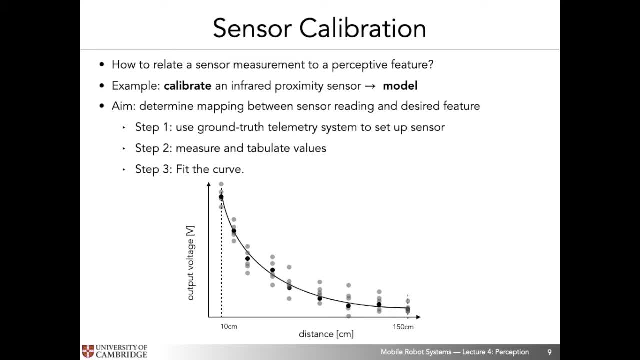 feature, And it relies on three main steps, where the first step uses a ground truth telemetry system to set up the sensor. The second step then consists of measuring and tabulating these measured values with respect to the ground truth values that we used in the setup of step. 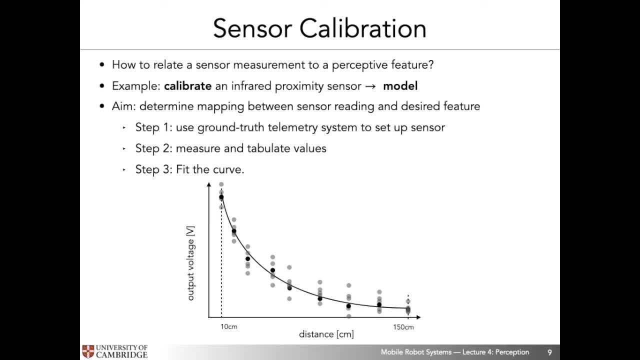 one. And the third step consists of actually fitting a curve to create a more compact representation of the relationship between sensor output and perceptive feature. So, in order to create these compact representations of these measurement feature relationships, there are different ways we can think of doing this. One way is to think about 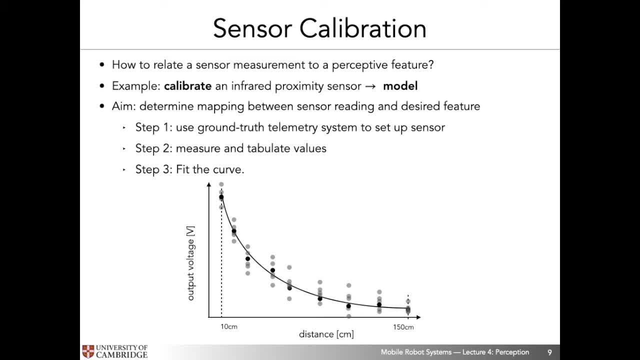 creating a curve, or fitting a curve to the set, the collected sensor measurements, And this curve would then ideally correspond, in the case of infrared sensors, for example, to a signal whose intensity decreases with the square of the distance, Because this is something that we know from first principles: how infrared proximity is supposed to behave. right, And you? 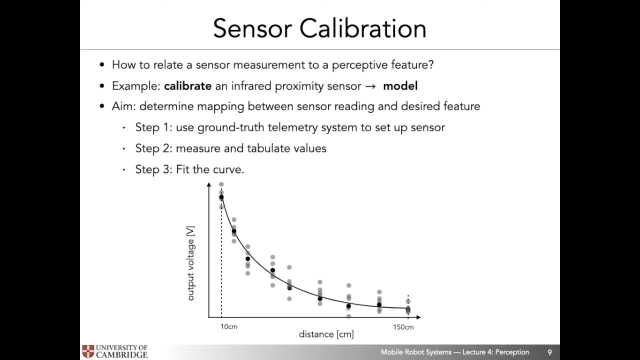 can see here in this plot that I'm showing you, as expected, that the sensor will actually not return the same value for each distance. Now, why is that? Well, if we go back and think about some of the things I talked about in the preceding lectures, 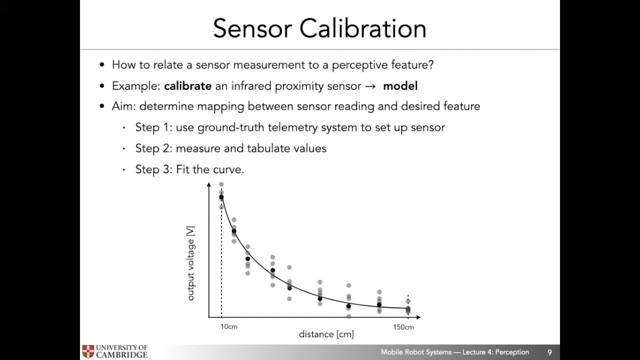 key items I kept on stressing was that in any robotic system, there will be uncertainty, And this uncertainty arises due to malfunction or cheap production of the sensors, but also to uncertainties and unmodeled or undermodeled artifacts in the environment. right, So it is. 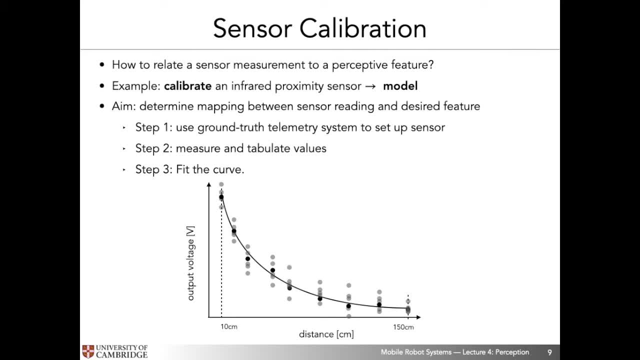 quite normal that if you place your sensor in front of a wall at a fixed distance and you don't move it, repeated measurements will not always be the same. There happens to be noise. Now, one of the key questions that calibration and sensor models deal with is exactly how to deal. 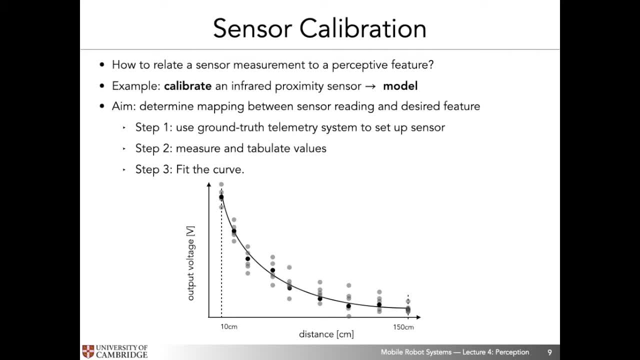 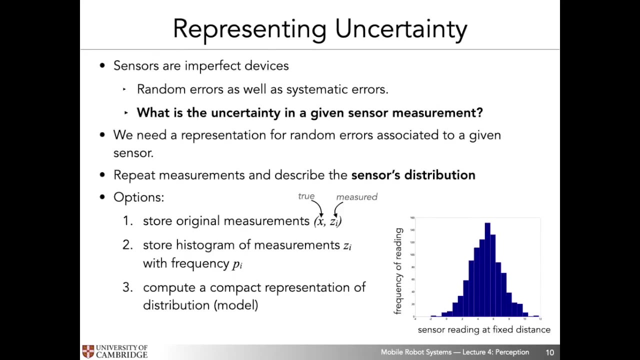 with this uncertainty, Because dealing with this uncertainty is really crucial to effectively and efficiently solving the perception problem in robotics. So, as established, sensors are imperfect devices and it is important that we have a method or methodology by which we can represent sensor uncertainty. So we know that errors occur due to randomness, so unknown, or 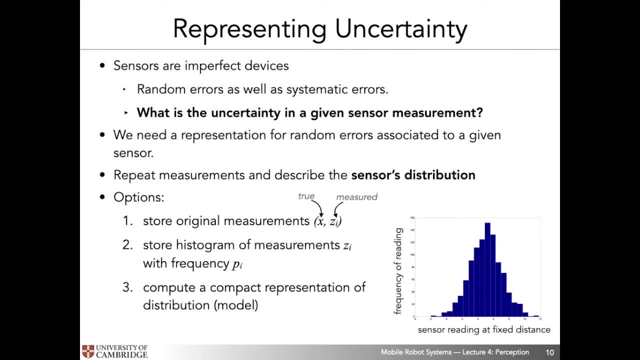 unmodeled reasons as well as systematic errors, And the quest that we're going to try to follow now is the quest of trying to represent uncertainty in a way that we can exploit it and use it in our perception algorithm. So the first thing that we're going to try to do is we're going to try to 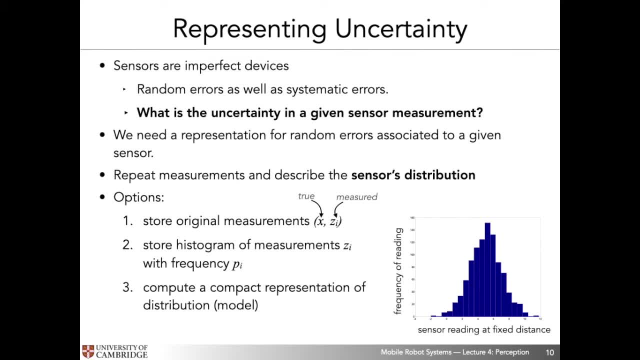 do is we're going to try to exploit it and use it in our perception algorithm. So the key thing here is representation, And there are several ways by which we can create representations for sensor uncertainty. So, since we want to infer features for measurements, we need to know how much we can. 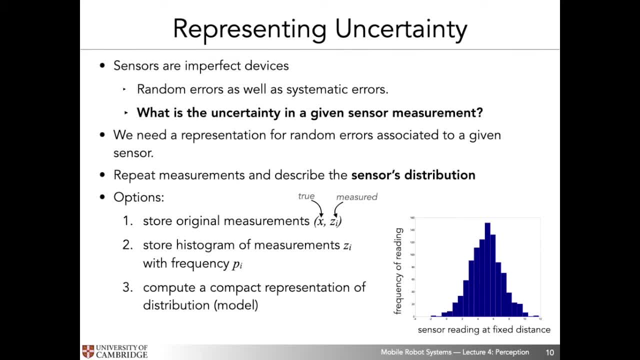 trust this inference And we need to represent this uncertainty because we need to know what the confidence is in interpreting what the sensor is telling us. And the key question we're going to ask is: what does the sensor's error distribution look like? So the process we're going to follow, 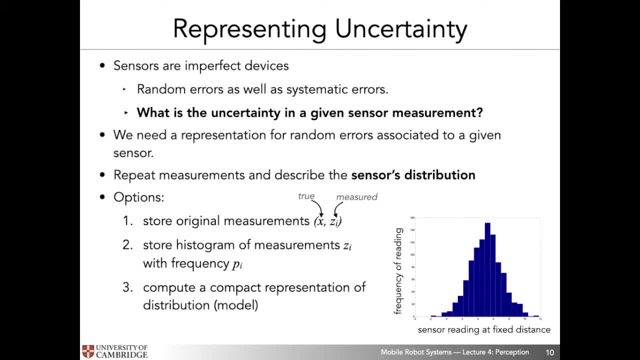 is, we're going to do measurements in a controlled setup, as described in the previous slides, And then we're going to create a model. Now there are three different options for creating this uncertainty model. The first option consists of storing all original measurements together with the true 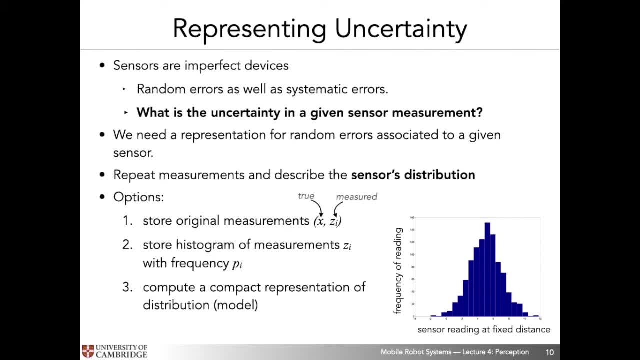 ground truth measurements. So the measured values are Z, underscore I, for all measurements I and the true ground truth value is X. The second option would be to store a histogram of measurements Zi with a frequency Pi, And the third option would be to compute a compact representation or 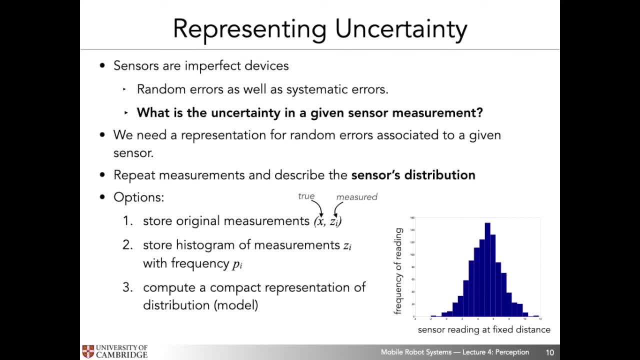 model of this error distribution. Now, the problem with option one is that clearly this is a lot of data, And what do we do if a new value is measured? How do we add that data to our table, etc. So this is not a very 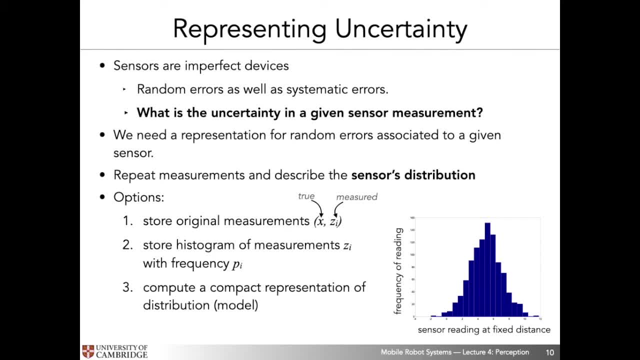 elegant or efficient way of modeling error distributions. The problem with the second option is that a histogram is also a discrete collection of data as the first option and is still can be very approximative depending on the bin sizes that we use, So a little bit more practical than the 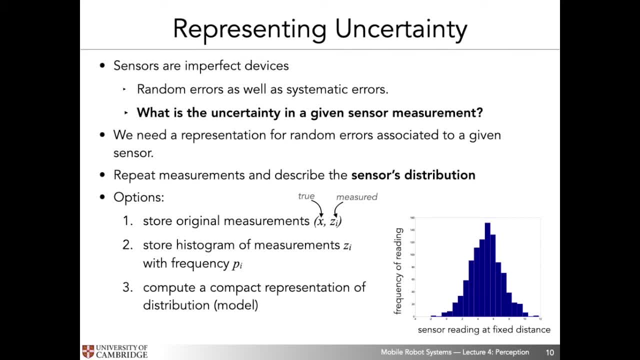 first option, but still not ideal. And the problem with the third option is, although this is definitely the go-to way of doing things, these days models can tend to be too general right. So we look, we tend to choose a template model with perhaps some parameters that we're going to try to. 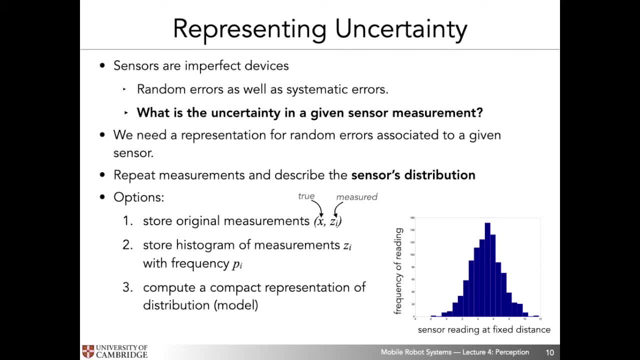 fit, And then this template model might not be the right one. So, for example, if we choose a Gaussian, a Gaussian would only have one mode, and perhaps the underlying distribution actually has two modes, is bimodal, or perhaps it has a heavy tail, or it is skewed, etc. And these are things that 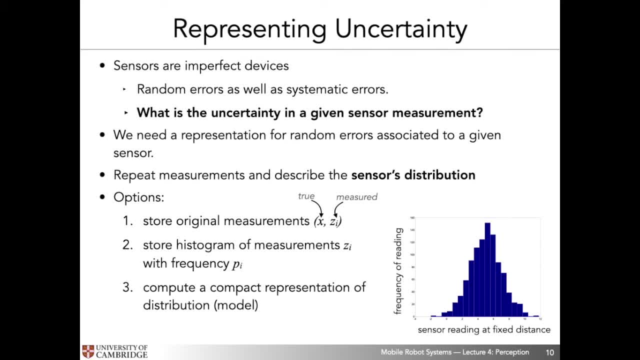 depending on which template model or default model we choose at the outset, will affect the accuracy and efficiency or applicability of the model that we end up fitting to the underlying data. So now let's have a look a little bit more at an example of how we would 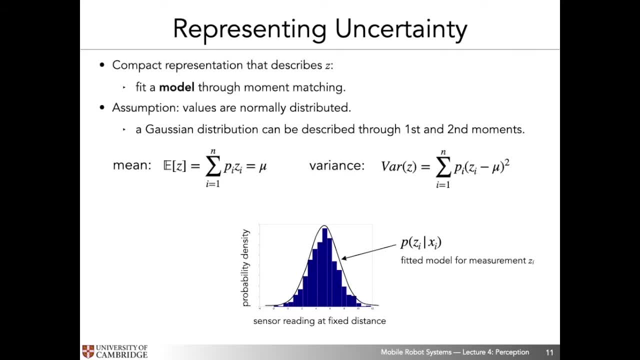 do this model fitting. So what we're going to do here is we're going to represent uncertainty through parametric model, and the process here is we're going to choose a template model. in this case we're going to choose a Gaussian, and then we're going to match the Gaussian moments. So the first operation: we're just going to try this well, so maybe we could do less function. if I take the model, for instance, to the bottom arched edge, that would follow the details over here as well as methodically just taking the model from final model into my tears. 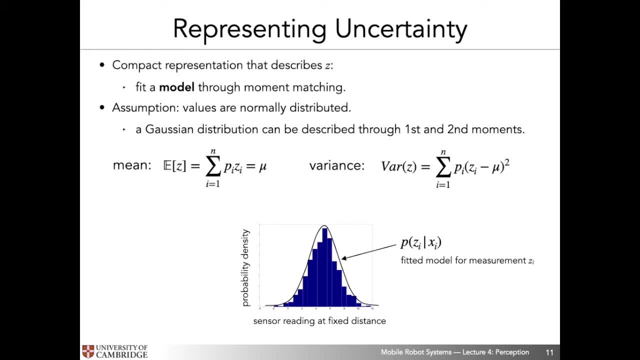 first moment here is the mean and the second moment is the variance And clearly, since we are choosing a Gaussian as our underlying model, we're making an assumption that our values or error distribution is normally distributed right. And the empirical formulas for the first and 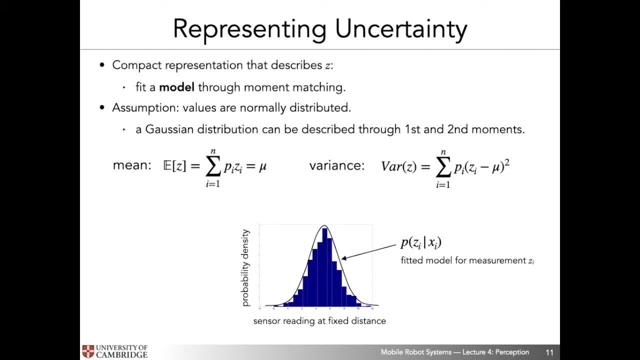 second moment are given by these two equations. So we have the empirical mean and the empirical variance where our z's underscore i's. here are the measurements that we take right, And so we can, given that we know we've completed our measurement campaign, we can then very easily 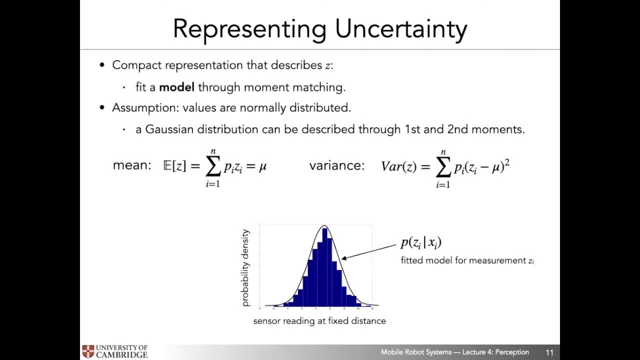 compute these two empirical values right Now. once we've got those two modes and we have our mean and our variance, we can actually plot the curve for our Gaussian. We can even fit it onto the same panel as our underlying distribution. Here I'm showing you a histogram plot of 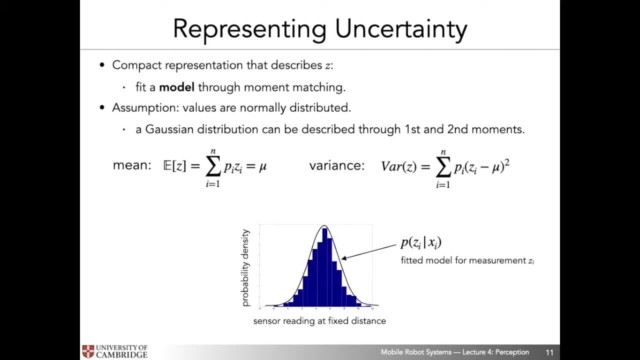 variance. And here I'm showing you a histogram plot of variance. And here I'm showing you a of variance. And here I'm showing you a histogram plot of variance. And here I'm showing you a true collected data. And you can see now that we have a model that looks relatively plausible for 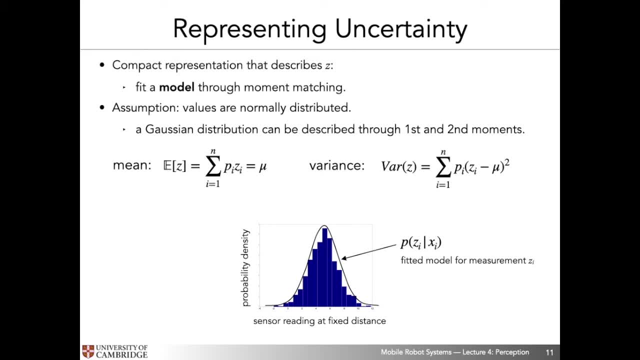 the underlying data. Now, what does this probability distribution function tell us? Well, what it is telling us is, or the question that it is answering, is: what is the likelihood of obtaining a measurement z i, given that I know that the sensor is placed at a distance x from a given? 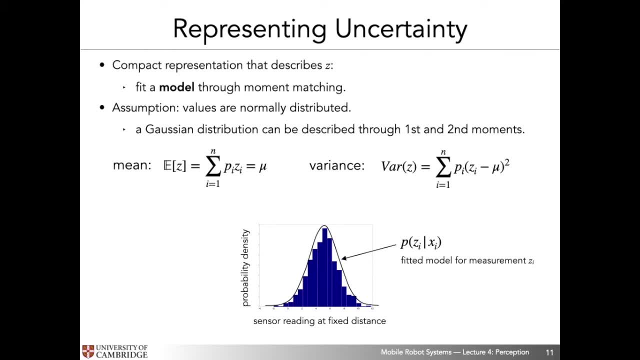 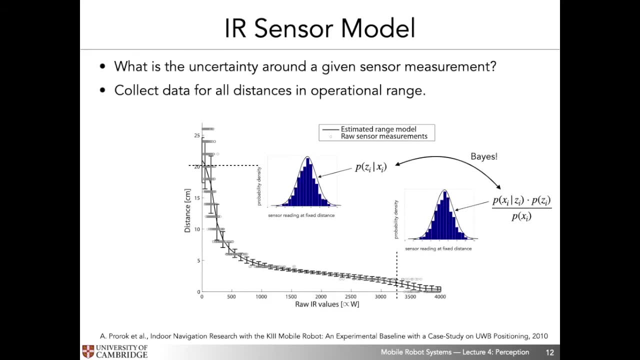 object, right? So that is what this probability density function is telling us. okay, Now let's have a look at how we can make use of this sensor model. right? And the question we really want to answer is: well, what is the uncertainty around a given sensor measurement whereby we actually 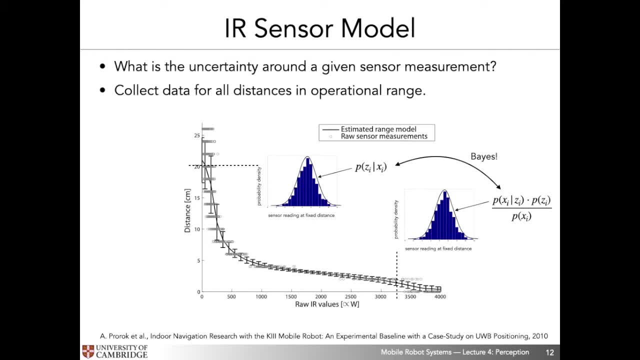 want to know, in the case of perception, perhaps not so much what the likelihood of a measurement is, but perhaps we would like to know what the probability is of being at a certain position. right, So let's think a little bit about how we would make that. 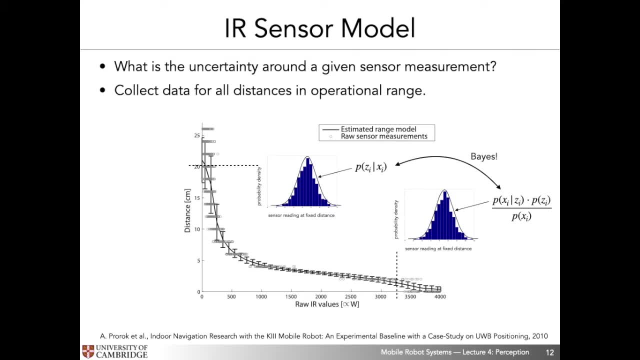 transformation from this one question to the other question. So let's have a look at this panel here. What we can see here is, on our y-axis, we're taking measurements at about 14 distinct distances, at roughly two centimeter intervals, And we're bunching these measurements. 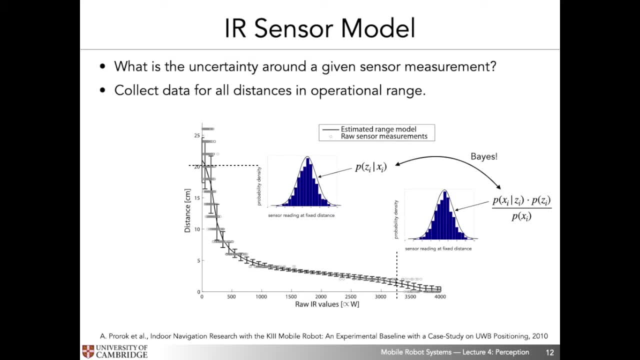 together that we took with this infrared sensor for each of the distances used in this measurement campaign. Now if I take a slice through any given one of those distances on my y-axis, we get the model that I showed you in the previous slide. 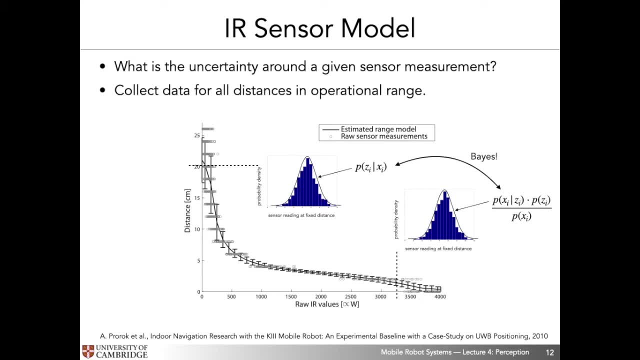 which corresponds to the probability density function. that describes the likelihood of a measurement z conditioned on a distance x, right? So, knowing that I took a measurement at, say, 15 centimeters, this is the distribution of errors I would expect. right? So that's what? 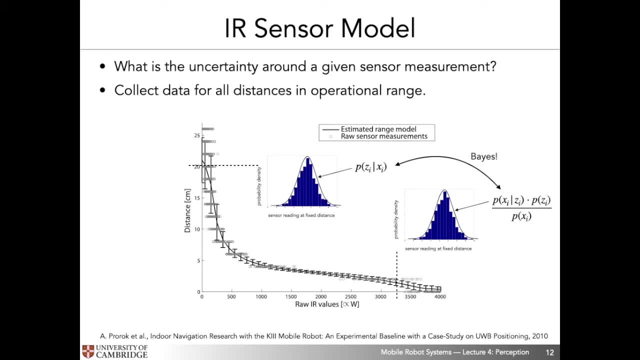 I'm going to do So. if I take a slice through my y-axis returns me. Now what if I want to answer the opposite question? So what is the likelihood of a given distance x i, given that I take a given a certain measurement right? So this is not an unreasonable question to ask, because perhaps 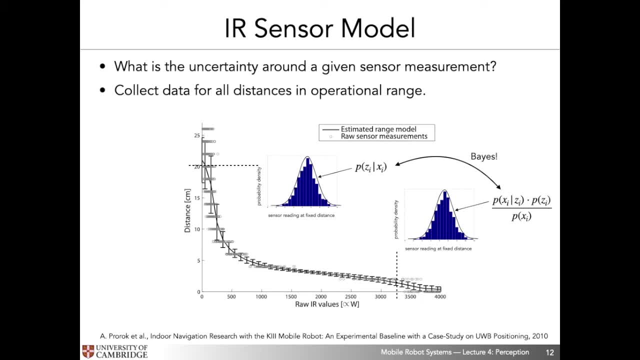 your robot is moving along somewhere and it takes a certain measurement. And given that one single measurement, you now want to answer the question. well, what is the likelihood that I'm 10 centimeters away from a given wall right- And that is the utility of asking this question- the opposite way around. 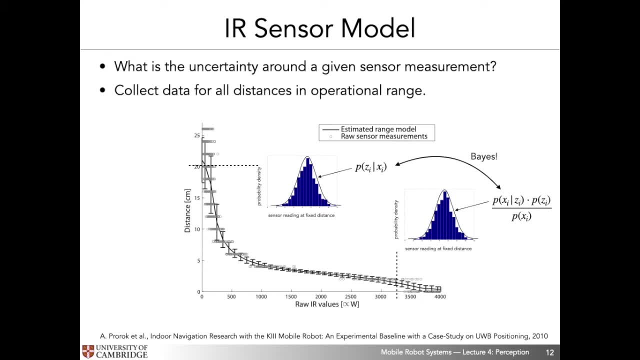 Now we might be tempted to take a slice of the graph in the other direction. However, Bayes' theorem actually tells us that we can only use this data directly to infer p of x given z if the sum over our pz divided by px is 1 for all. i's meaning that we have a uniform. 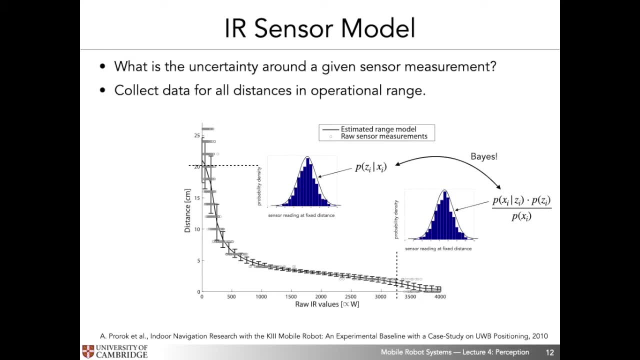 distribution over any measurement right. So in other words, all measurements z, i for any given x or for a given x are equiprobable, And this is not true in general. So a counterexample would be: you're in an environment where you see a wall much more frequently from a specific distance than from another. Hence, if you 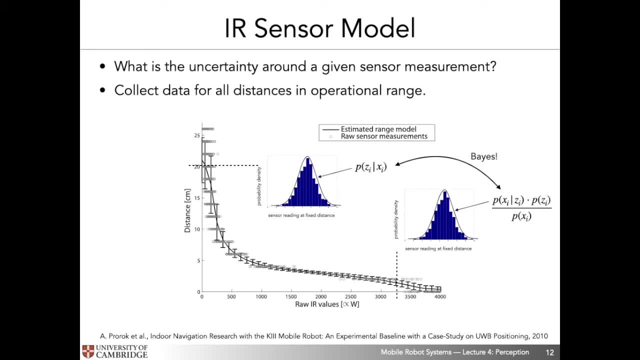 slice through your data vertically, you'd get a skewed distribution that would need to be scaled by p of x. Hence the takeaway message here is that px of z is, in general, highly dependent on the given environment. So, to summarize, to formally represent the model p of x given z, we need: 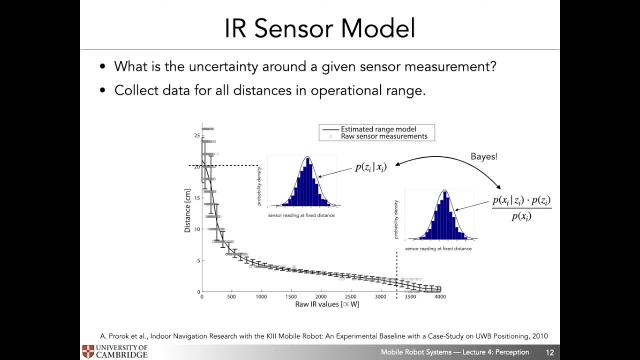 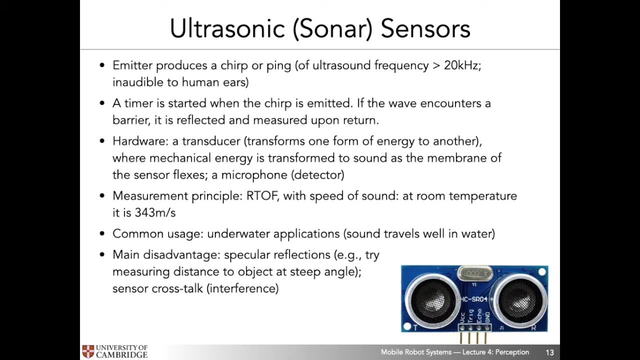 Bayes, as well as values for pz and px, for all i's. So now let's talk about another type of sensor, so ultrasound or sonar sensors. So, first of all, how do sonars actually work? So sonars are a type of sensor that can be used to measure the temperature of a given environment. 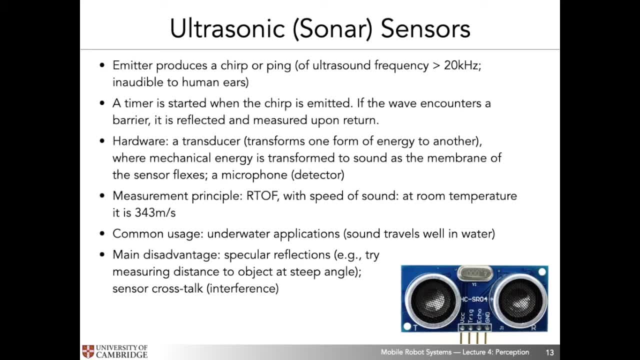 Sonars are active sensors that consist of an emitter and a detector. The emitter produces a chirp or a ping of ultrasound frequency. This sound then travels away from the source, and if it encounters a barrier it'll bounce off it, So it'll be reflected and perhaps it will return to the 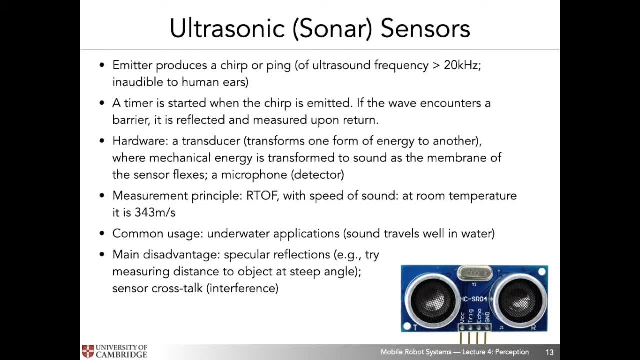 receiver. So in this case, because we're talking about sound waves, receivers are generally microphones, So if there's no barrier or if this emitted sound wave is not reflected, it doesn't return in general, and nothing will be detected at the receiver end. 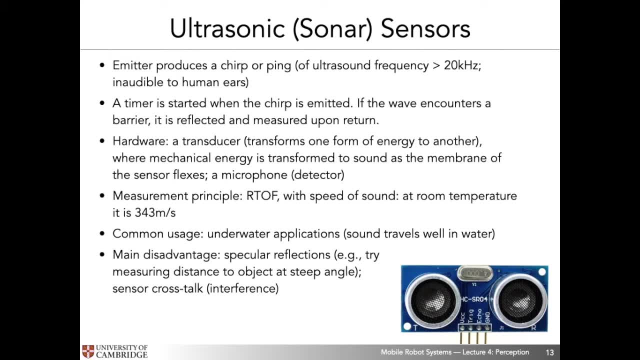 So if the sound does return, then the amount of time it takes for it to return can then be used to calculate the distance between the emitter and the object or the barrier that the wave encountered and made it reflect and return to the receiver. So this is how we would actually 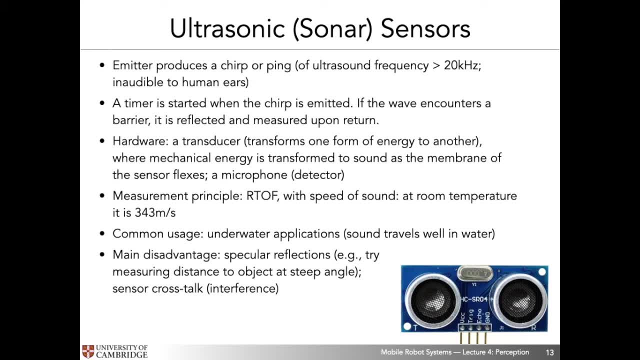 implement such a system. So if the sound is not reflected, it doesn't return, and if it's not reflected, it doesn't return. So a timer is started when the ultrasound chirp is emitted and it is stopped when the reflected sound wave returns. So this resulting time then is multiplied by the. 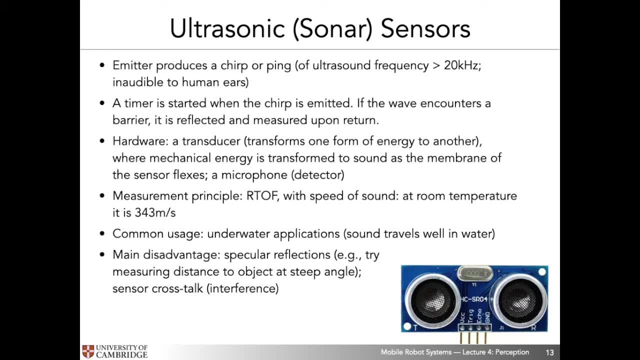 speed of sound and divided by two, because the sound traveled to the barrier and back, and we're only really trying to determine how far the barrier away is from our emitter. So it's only a one-way distance that we're interested in. So a very simple measurement principle. 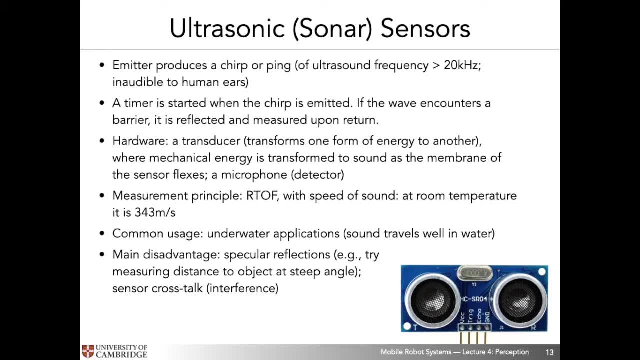 Now, the main disadvantage of ultrasound sensors is that they're dependent or they're sensitive to specular reflections, right, So this can produce cones, and the sensor readings are generally interpreted as arcs and not as point measurements, And this can introduce some complexities in 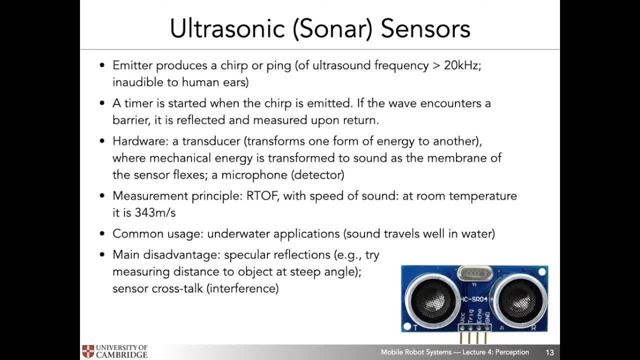 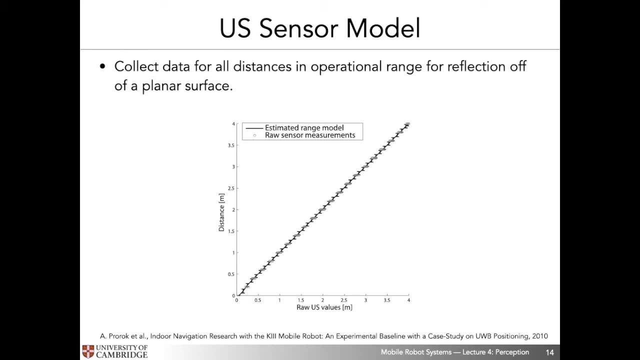 the values that are actually being returned to the receiver device. But in general, ultrasound or sonar sensors are very benign because they have very linear characteristics, given that we're measuring time of flight. So this is some data from an actual measurement campaign and you can see how beautifully linear the raw ultrasound values. 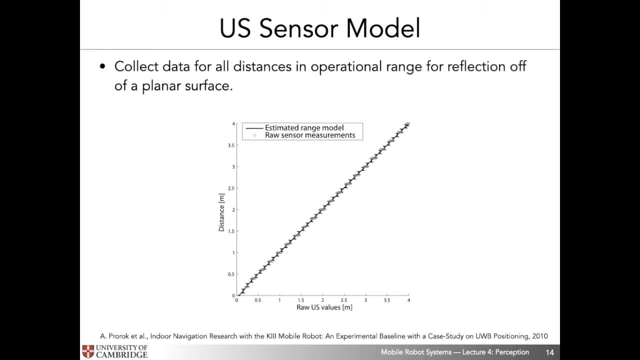 behave with respect to their ground truth measurement distances, And on top of that you can see that the variance is very small. So linearity and very small variance are two very attractive properties for any given sensing modality, because it means that there's little. 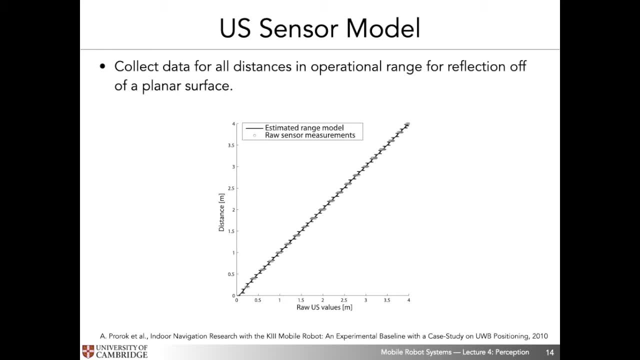 uncertainty in the values that we're receiving, and we can use those directly to infer the perception features that we're interested in. Now, there's a small caveat here, obviously, and that is well: what kind of environment was this measurement campaign taken in? And clearly, if you? 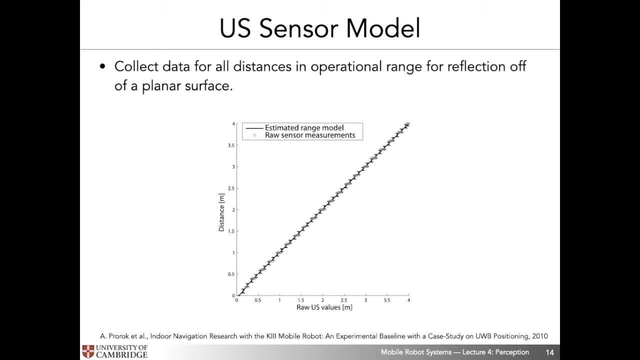 look at the underlying paper here, you can see that this control setup was very benign, so there was only one surface distance. And then, of course, there's also the fact that the measurement was very smooth and the robot was actually facing it. So no ruggedness, no cones, no sharp acute. 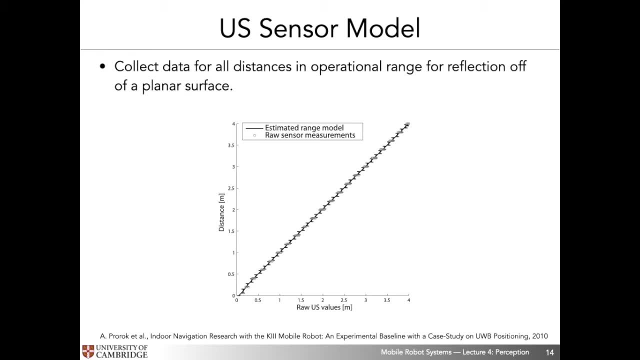 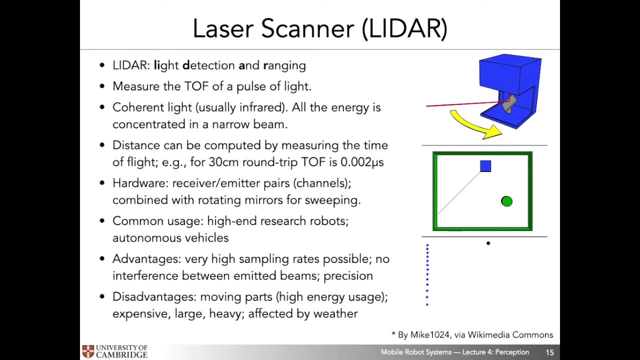 angles, and that definitely does impact the values that are being returned to the sensor. So now I'd like to look at another type of sensor, which is the laser scanner, or otherwise known as a LIDAR, which stands for light detection and ranging. So LIDAR is just like. 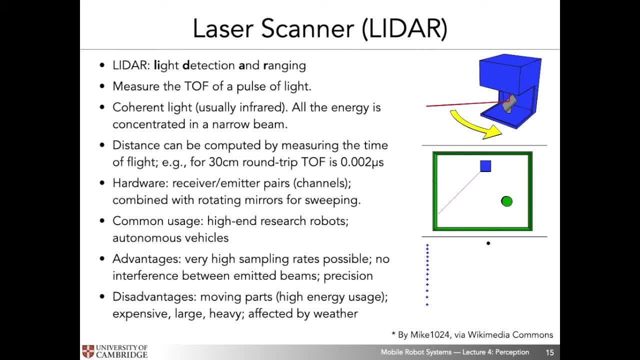 a laser scanner, but it's a laser sensor. So it's a laser sensor and it's based on the simple measurement principle of time of flight. In the case of our LIDARs they're based on a pulse of light right And the modality here is coherent light, so usually infrared. where coherence means, 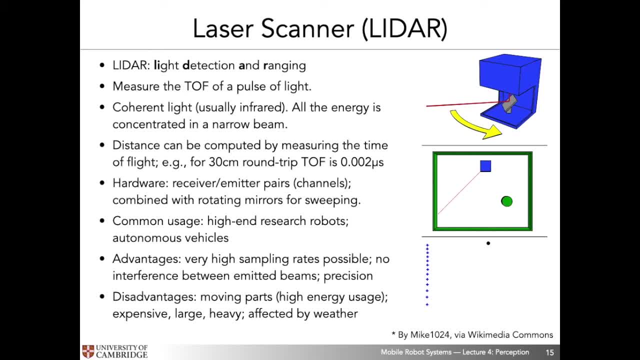 that all waves are of the same frequency and the same phase, So the start of each wave is at the same time, And this means that all the energy is concentrated in a narrow beam. Then, with the time of flight, the distance is computed by measuring the time of flight. For example, if you 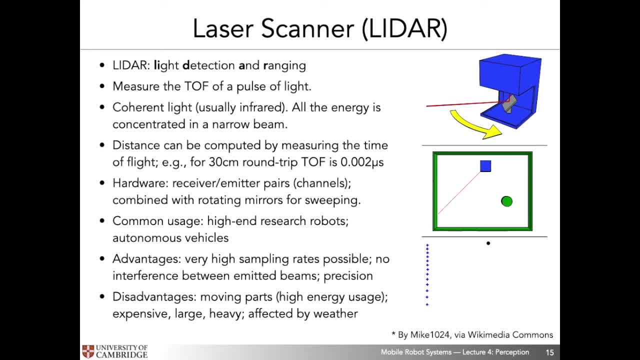 look at a 30 centimeter round trip, the time of flight would be 0.002 microseconds, since we know the speed of light. The hardware consists of receiver-emitter pairs combined with rotating mirrors for sweeping to give us more field of view. right, And the common usage for LIDARs is 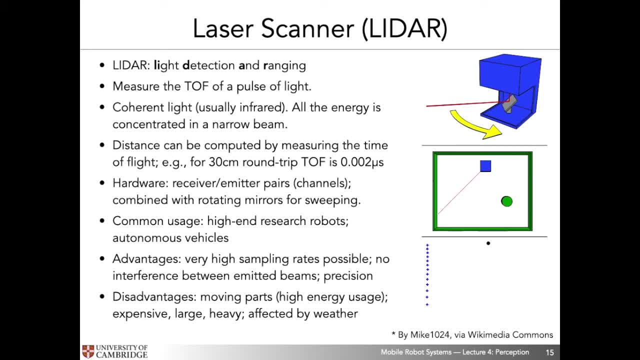 really high-end research, robotics or actual commercial applications such as autonomous vehicles. And this is mainly due to the price range of LIDARs, and we'll talk a little bit about that in a few slides down the road. So the advantages of LIDARs, despite their high price. 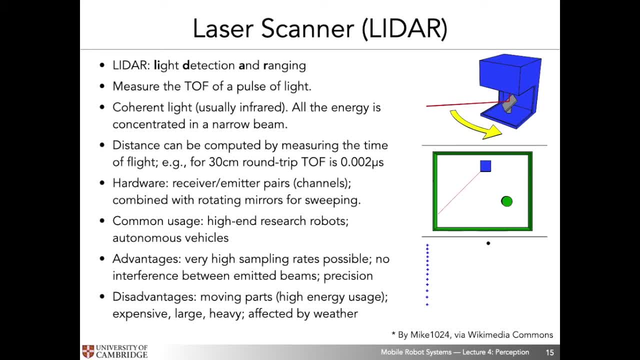 and more complicated construction is that they are able to deliver very high sampling rates and that there is no interference between the emitted beams. So, ultimately, they're very precise sensors if we know the conditions, though the environmental conditions that they're operating in, So they're able to deliver very high sampling rates and they're able to deliver very high. 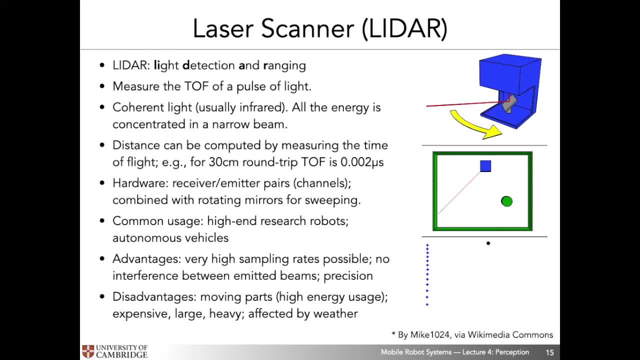 sampling rates. So the disadvantages, however, are that they rely on moving parts, And let me just see if I can play this GIF here. Yeah, so you can now see how the actual measurement principle functions with the rotating mirror to allow the laser rangefinder to increase its field of view. 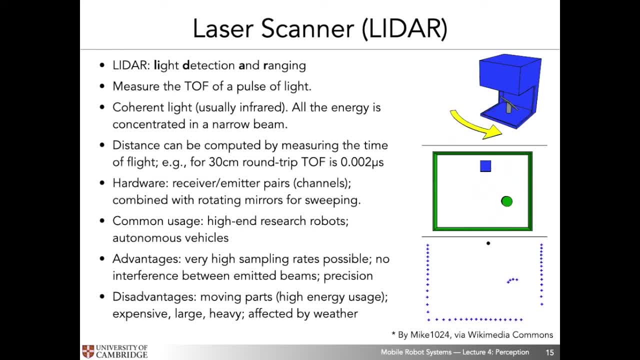 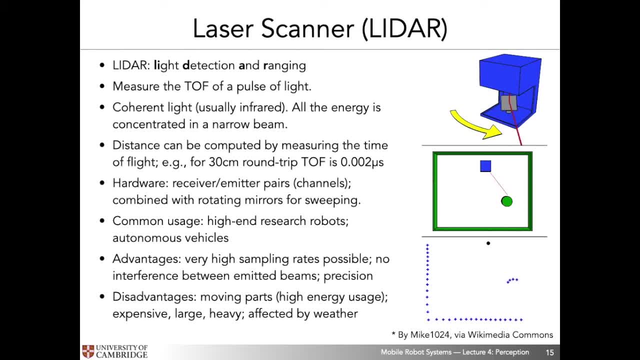 disadvantages of laser rangefinders, in terms of their efficiency for perception algorithms, is that they're heavily affected by weather, So light is not only reflected by objects, but it's also reflected by dew or rain or fog or strong incumbent light sources. All these 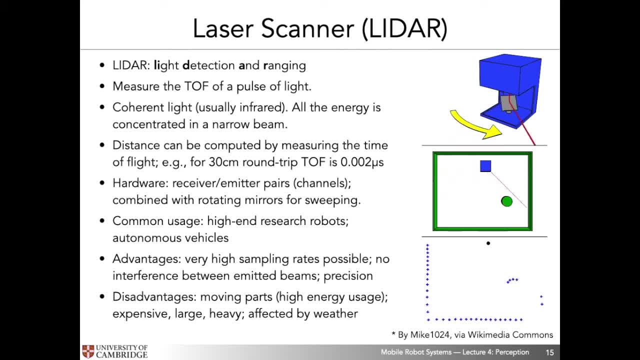 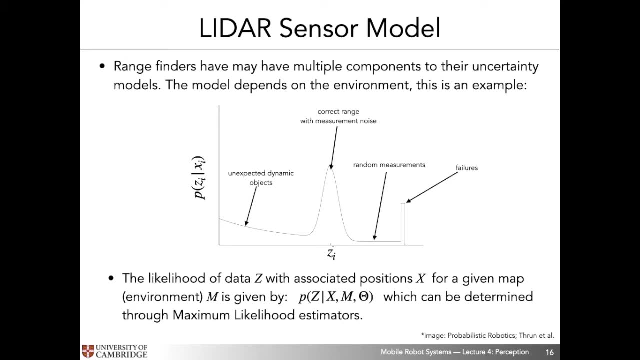 aspects can heavily impact the accuracy of the measurements that are being returned to our receivers. Okay, So, as before, we're going to have a quick look at how we might want to develop a sensor model for laser rangefinders. Now for a LiDAR. what would a feasible 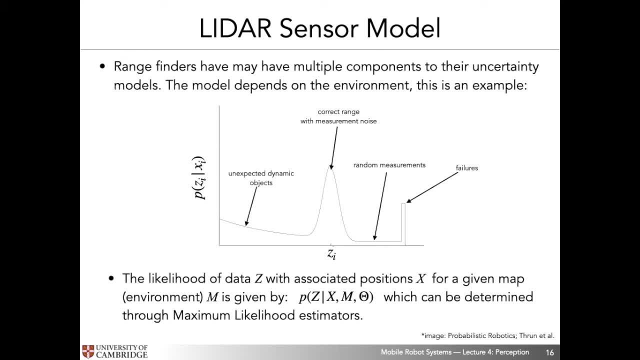 sensor measurement model look like? Now, there's not just one answer to this question. There are many possible approaches we could take to develop a sensor measurement model for laser rangefinders, And the one I'm going to just briefly introduce here is one example that was first introduced in. 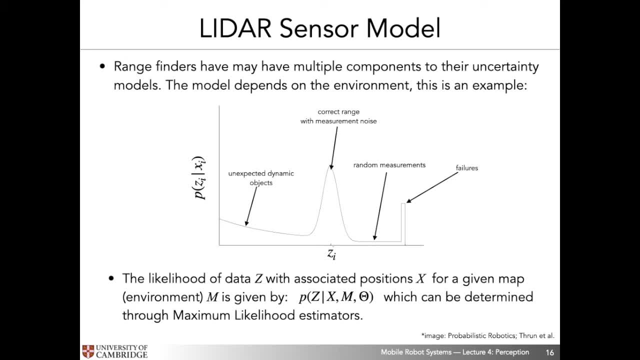 Truen's book. So the first thing that we want to do when we're dealing with a sensor is we want to apprehend the different types of behaviors that a sensor might be in in a certain environment. So what types of behaviors are expected from real world laser measurements in any possible? 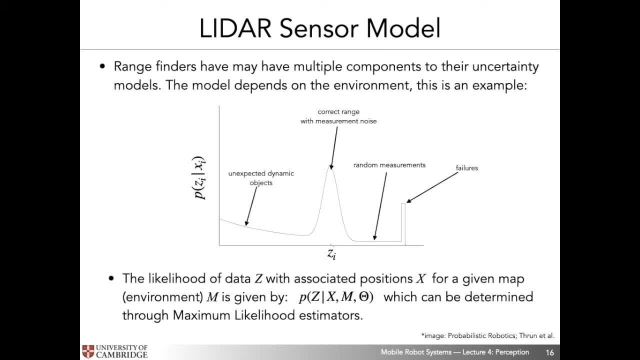 environments, right. And then we want to apprehend the different types of behaviors that a sensor might be in in a certain environment. So what types of behaviors are expected from real world laser measurements in any possible environments, right. And then, once we've kind of brainstormed through, 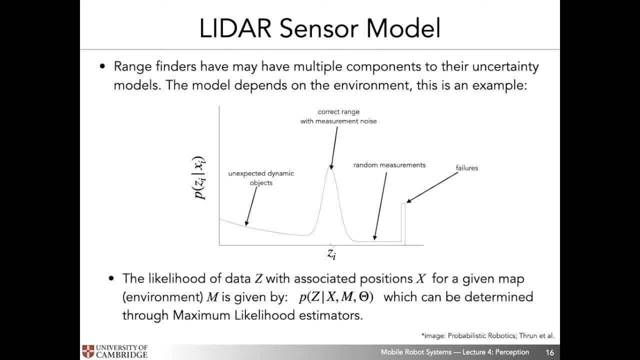 possible behaviors. we would list them And we might want to compose a model that consists, or is able to model, these various behaviors that we're going to be expecting. Okay, So let's try to translate this rationale into a sensor model. So the first type of behavior we might want to model, 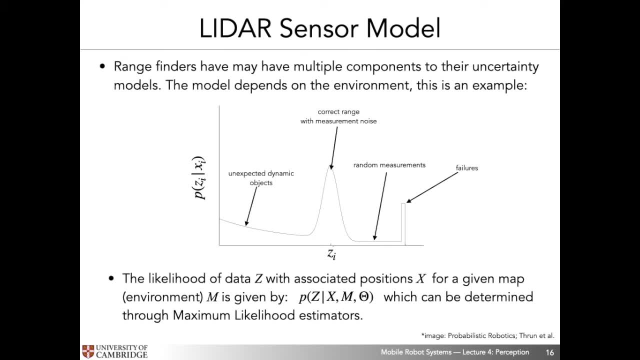 for laser rangefinders is the event of unexpected nearby dynamic objects, right, And this is called a sensor model, right? So that's unexpected moving objects that are nearby, nearby the robot. Those would be modeled by this sensor model, right? And then the second type of behavior we might want to. 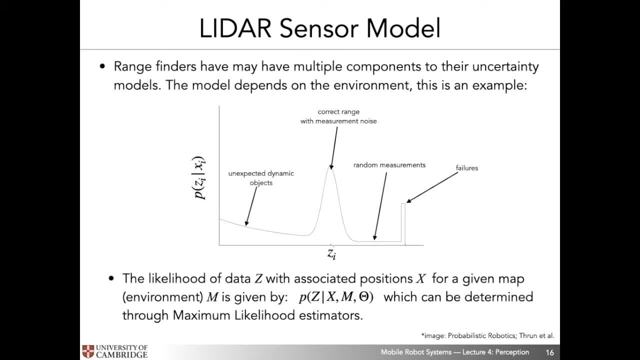 model is increasing likelihood of unexpected dynamic objects as we get closer to the actual sensor. Then we might have a standard Gaussian to model, standard random noise around the correct range, right, So that would be around our ZI, And then that was so. that would be our second mode. 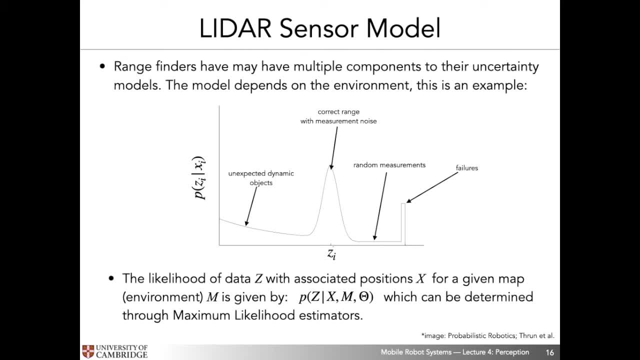 And then we might have a third mode, which here consists of a simple uniform distribution across our whole system. And then we might have a third mode, which here consists of a simple uniform dosto support, just to consider all unexplained measurements we might encounter. right, So no. 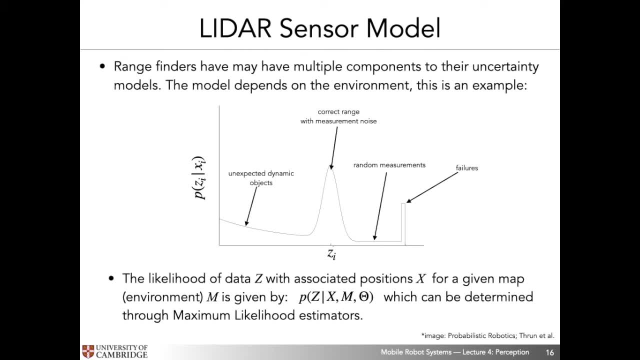 for no particular reason, any given measurement might h peson that we want to capture on the uniform distribution. And then, finally, we might have a fourth component that, taken, takes into account all failures, So sometimes that these would occur when an obstacle is missed altogether, For example when 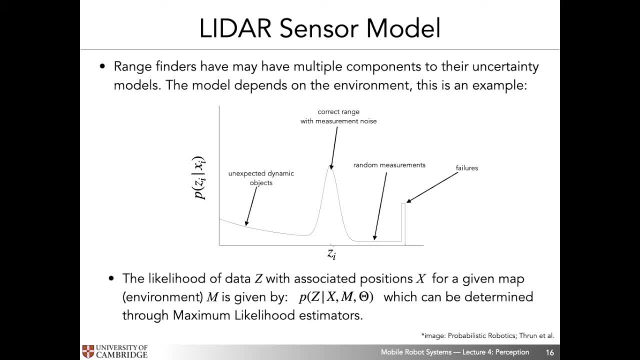 the lidar is measured. you use this as the交 sections here on the horizontal diagram in a Wilson diagram And then, after just brightening these rewind and measuring something at a very steep angle or when the laser rangefinder, when the object is trying. 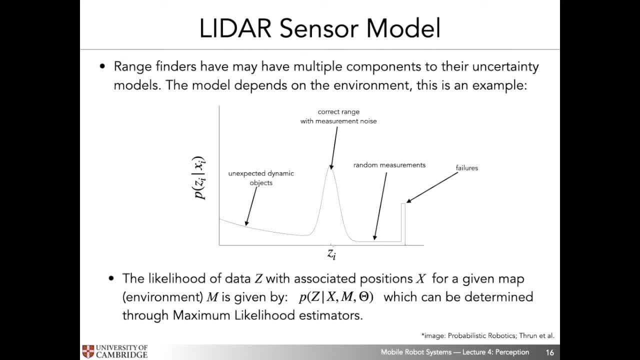 to when the laser rangefinder is trying to sense an object that has very high light absorbing characteristics, or when it's trying to measure something in very bright light. it might not be able to measure it and returns a failure, And this type of failure has to be modeled through the 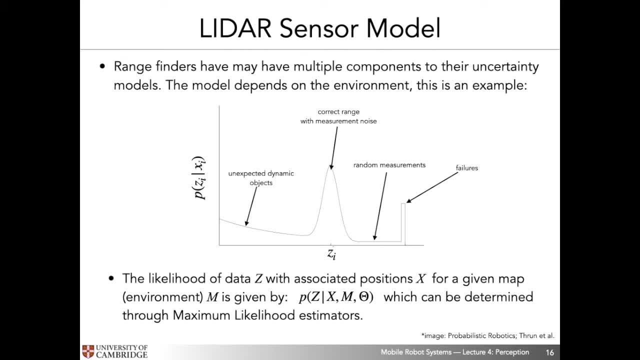 maximum range possible, given the sensing modality we have at hand right. So we have these four components we think are reasonable, given a certain general class of environments our sensor would be operating in and given that we know how laser range or how laser light operates in those kind. 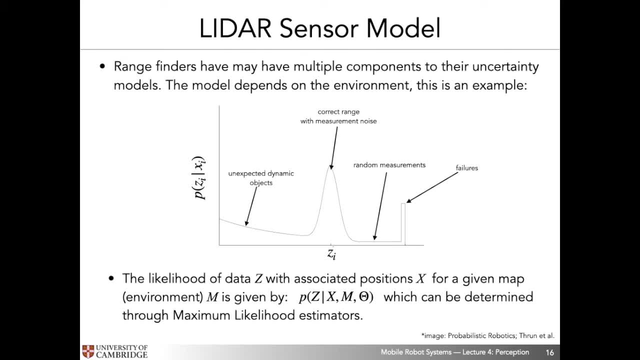 of environments right, And so we could go on to construct a template model right for these that combines these four modes, And then we would fit the parameters given underlying data and that would then give us our ultimate probability density function, much like we did for the more simple case of the infrared sensor. a few 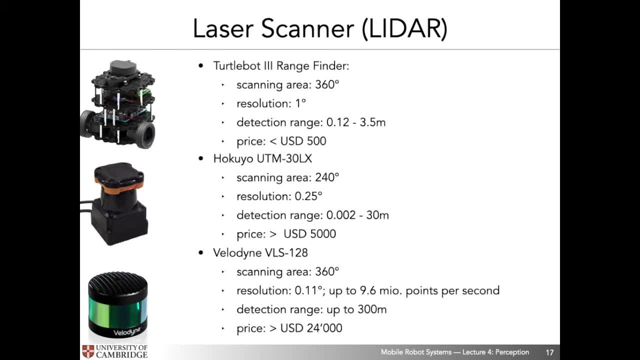 slides back. okay, So what kinds of laser rangefinders exist? And this is again an interesting consideration to make, because when you're building robots, price does make a difference. So, on the TurtleBot robots, which are the template robots, which are the laser rangefinders, which are the laser rangefinders which are the 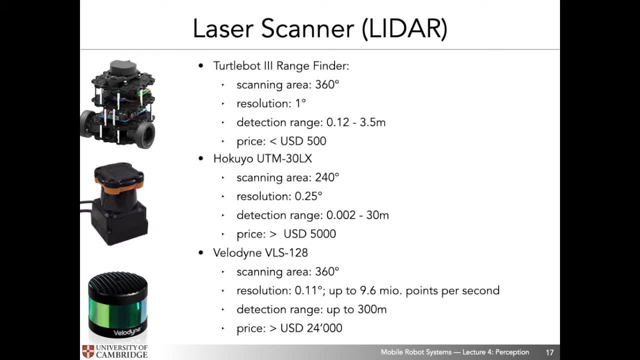 So on the TurtleBot robots, which are the laser rangefinders, which are the laser rangefinders, which are the robots, or the default, we consider in this course. we do also have a laser rangefinder. It's a very simple one in the sense that although it has a very wide scanning area- so 360 degrees visibility- it has a relatively low resolution, so one degree resolution. 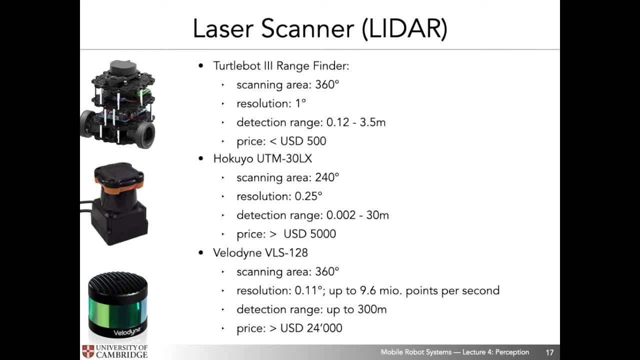 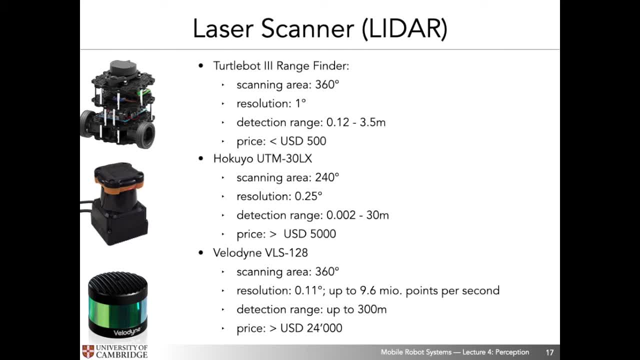 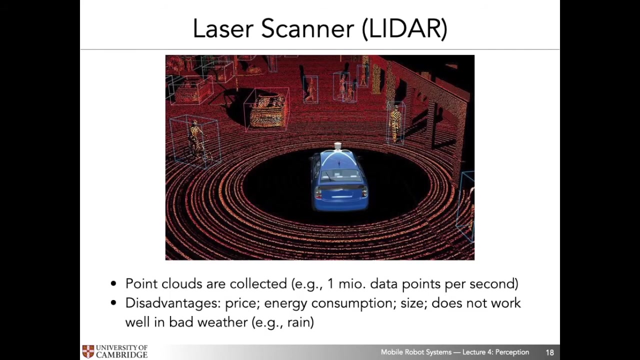 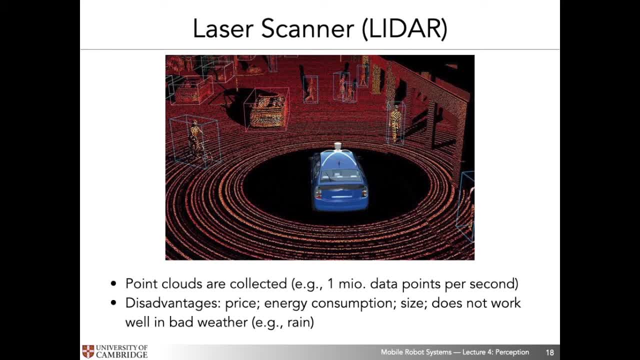 maps or dynamic maps of the environment at a very high resolution, by collecting point clouds and inferring the shapes of objects that these point clouds compose, right. so these point clouds, essentially what they give us, are depth information that is centered essentially at the origin of the laser rangefinder, and so 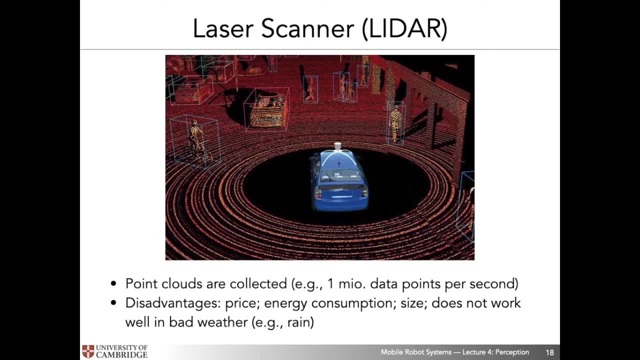 as you can see in this image here. this gives you a very rich picture of the kinds of things that are happening around your autonomous vehicle, and this is very useful for purposes of trajectory planning. now, one thing to mention here is that, although laser rangefinders do bring us, or give us, an, 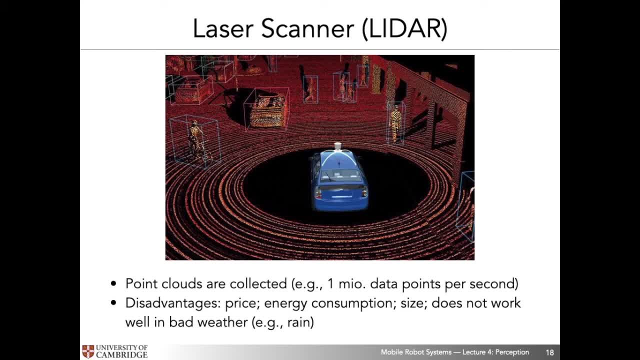 enormous richness in terms of information. they have a lot of downsides, the ones that I mentioned before, so the high price, the moving parts and especially their dependency on environmental factors, so weather and bright light, etc. which means that a lot of automakers today are actually not so. 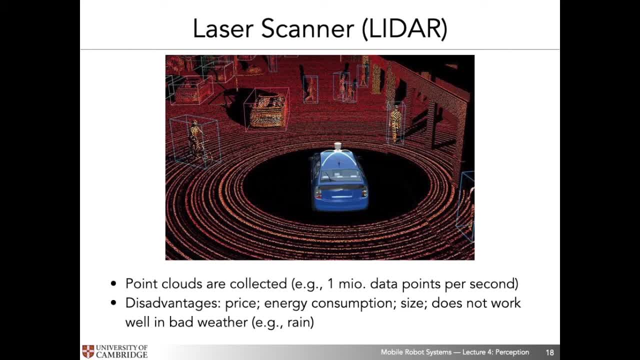 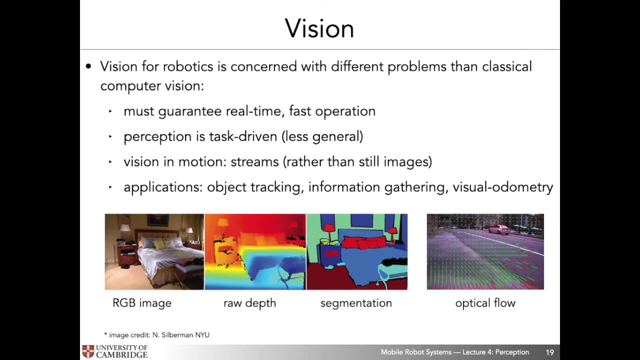 keen on laser rangefinders anymore, and you will actually see that the newest Tesla models and a couple of other automakers are actually not integrating laser rangefinders at all into their vehicle prototypes. so, moving on to a completely different type of perception, I just like to say a few words about vision. so vision is not at 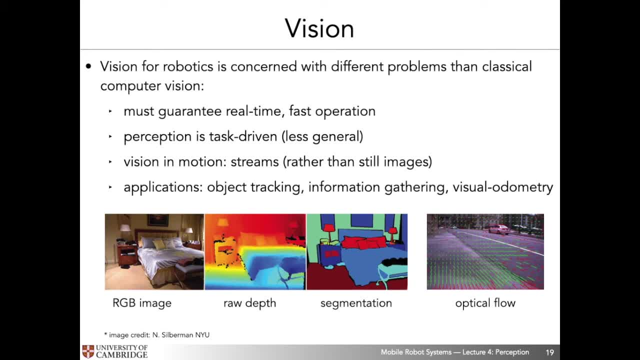 all going to be the focus of this course and we won't go into it in any in any depth at all, but I do want to just put it into the right context within the topics of this course. so vision for robotics is slightly different to vision in general. 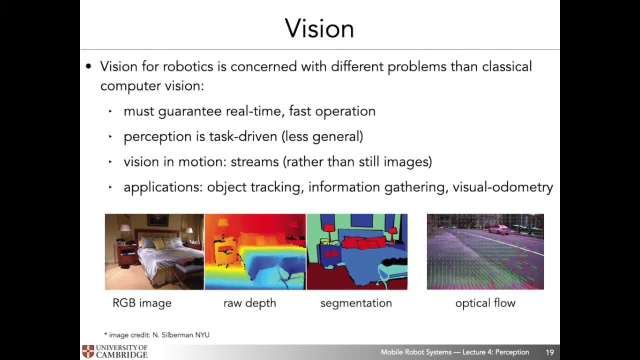 whereby in robotics we're actually interested in slightly different problem characteristics than classical computer vision would be interested in. so in robotics we're interested in certain guarantees, such as the real-time guarantees that vision algorithms could deliver, and of course they have to be able to operate very quickly. 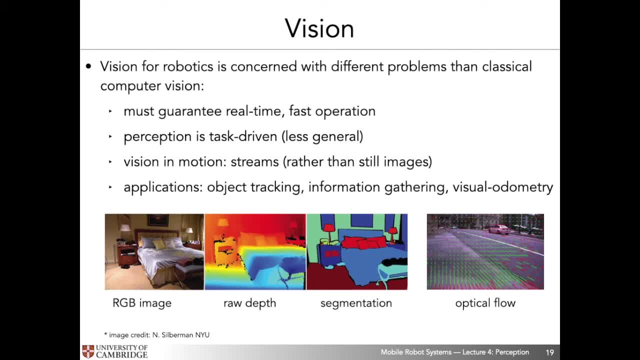 because we're talking about dynamic decision-making. when we use vision in robotics, The perception is task-driven when we use vision right. So we're not using vision in general to just classify anything arbitrarily. We usually use vision for very specific purposes. So, for example, we want to detect pedestrians and other cars. 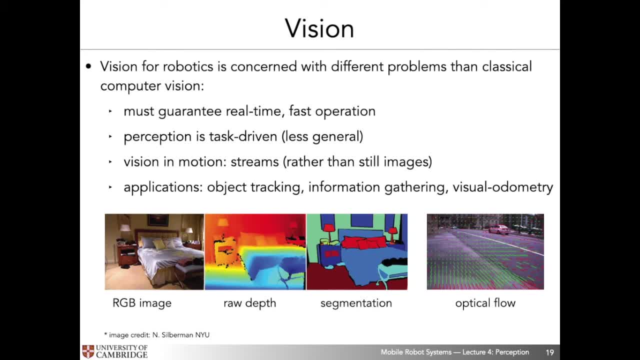 but are not necessarily interested in having classifiers that can detect any possible object that exists in the world right. So it's very task-driven the way vision is used in robotics. We're using vision in motion, right. So very commonly the cameras are placed on objects that are moving. 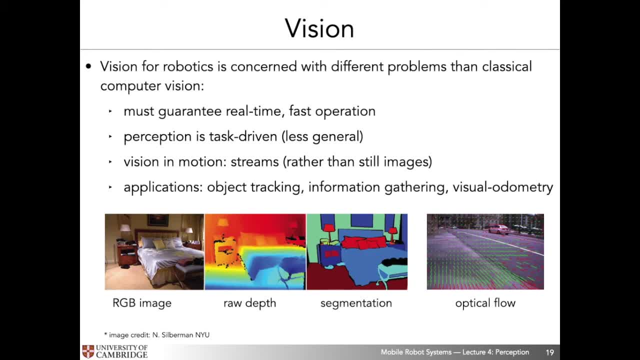 And hence we're using data streams rather than still images. So many of you who studied vision in machine learning classes are familiar with the vision databases that are just collections of static images. Well, we're really interested in streams, which produces completely different types of data sources and databases. 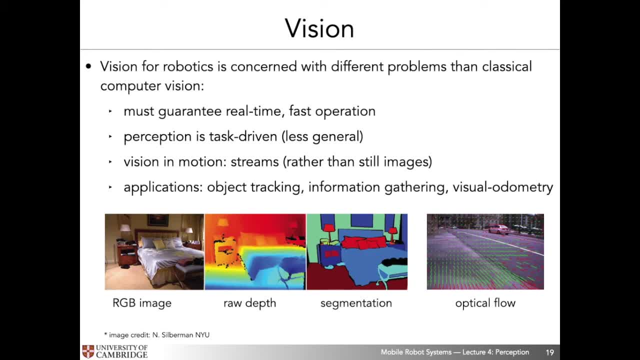 that we want to use, And so we would have to process in order to make sense of right. And finally, what applications do we actually want to solve once we have vision algorithms that work Well? common applications in robotics are, for example, object tracking. 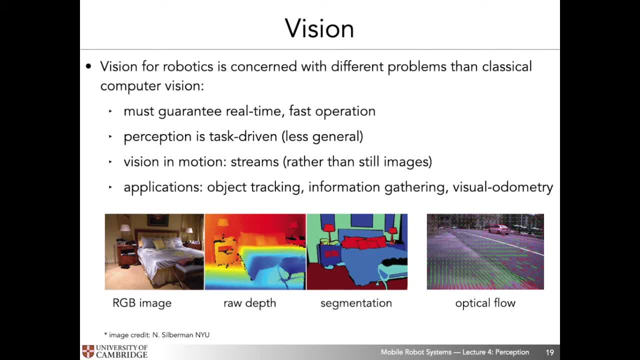 So you have a robot that is trying to hone in to a target, or because it wants to protect the target, or because it wants to follow that target for some reason. We might be using vision for information gathering, So you could think of environmental monitoring purposes. 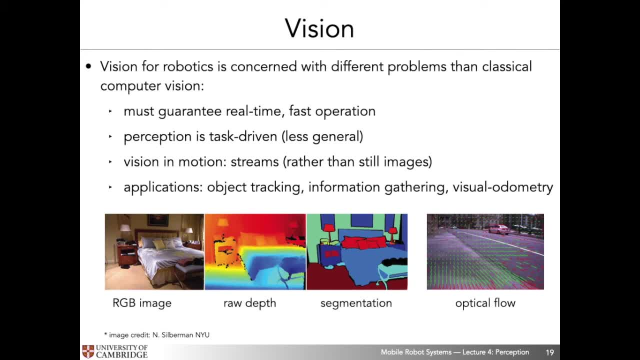 or a wildlife monitoring, and you would want to do those things in an autonomous manner, And visual odometry is actually also an application. that is perhaps more of a means to an end Visual odometry. what it allows us to do is actually it allows us to estimate positions. 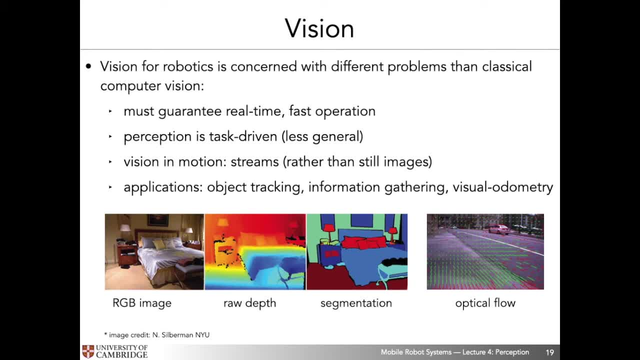 of autonomous mobile vehicles. So how visual odometry actually works, or otherwise known as visual inertial odometry- is by looking at objects, by looking at image frames as they come in in your stream, you can actually infer by how much your vehicle has moved. 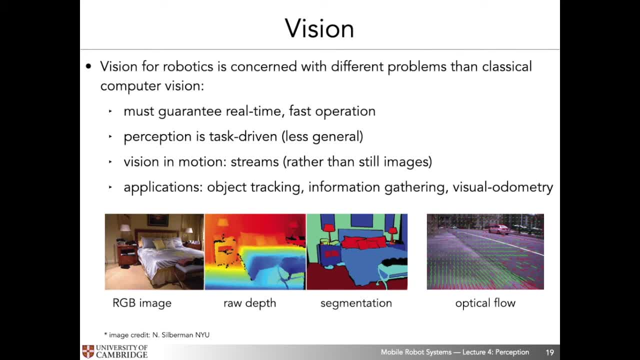 along your degrees of freedom by comparing neighboring frames- right And so this idea is very powerful and can allow you to use the idea of odometry- not using odometers but instead using visual input- right And so these are just a couple of ideas and applications. 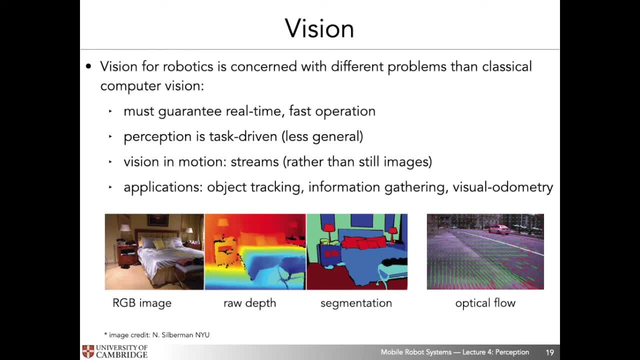 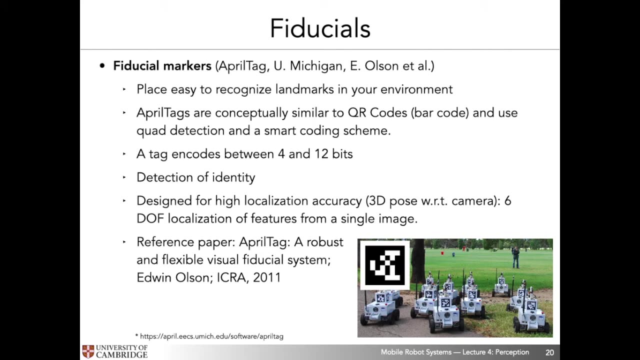 that are very popular within the field of robotics, through leveraging vision as our perception component. So now I just want to give you another example of a cool way of being able to sense robots or give robots sensing capabilities, And this component or idea I want to talk about. 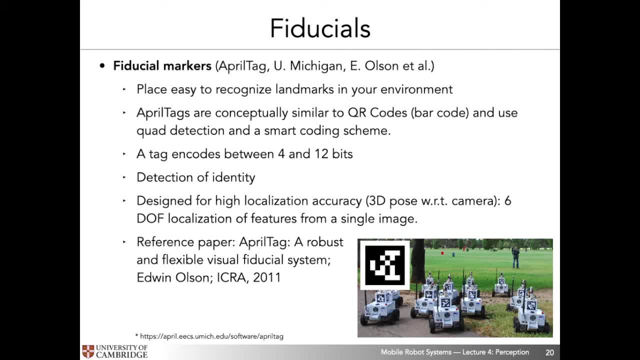 we refer to as fiducials. So what are fiducial markers? So fiducial markers. so fiducial markers were most recently popularized or made very well known within the robotics community by Edwin Olson at the University of Michigan, quite a while back actually. 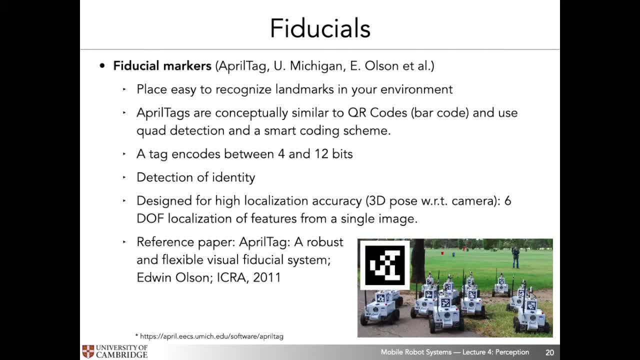 when he designed this thing which he called the April Tag, which is basically a piece of paper with a print on it that looks very much like a QR code, which allows you to easily recognize and position landmarks in your environment, right, And so these landmarks can be like landmarks. 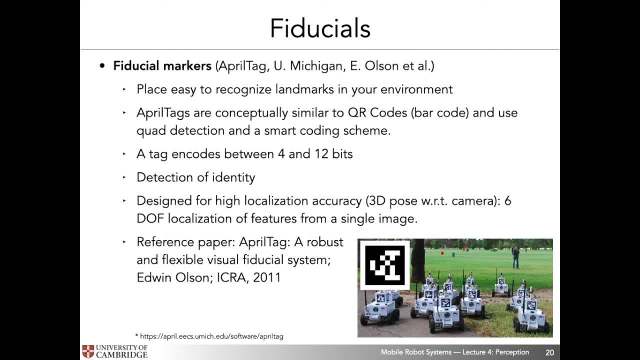 in the sense they're static beacons in your environment, but they could also be placed onto robots so that some robots can easily localize and position other robots that are carrying these fiducial markers right. And so the way these April Tags work are, in the sense. 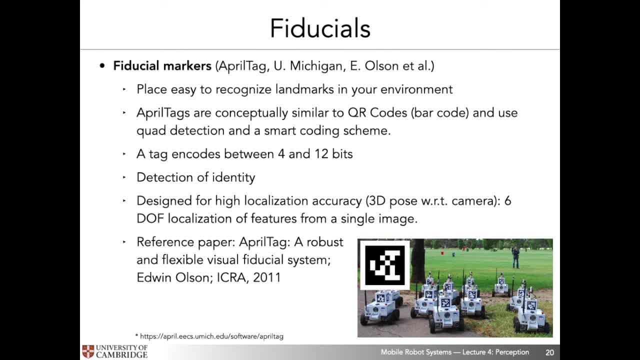 that they're conceptually similar to QR codes are that they localize the quad or they detect the quad, and the encoding in this quad or in the code allows them to detect the identity of the object and also use the bits in there to determine the 3D pose. 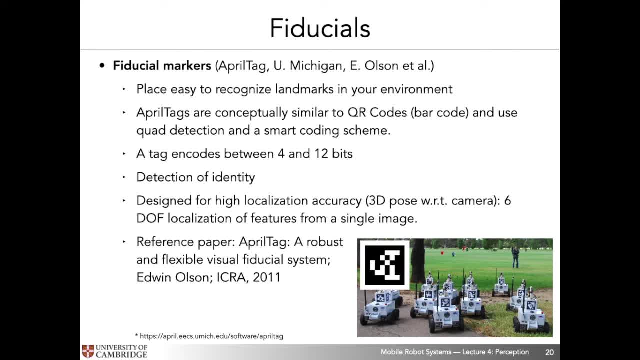 with respect to the camera that is detecting the quad right. So you place the print on an object, the camera that is on the robot detects it and then localizes it with respect to the camera position. So this is incredibly useful And for those of you who are interested in more details, 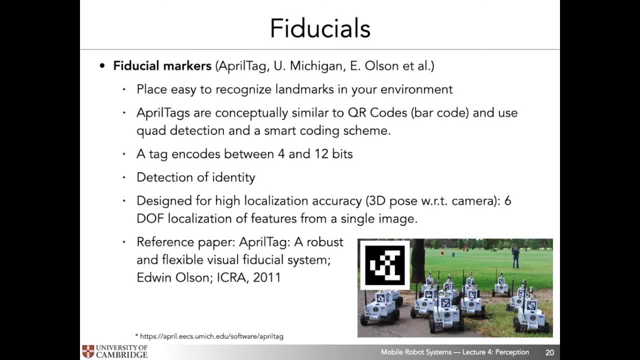 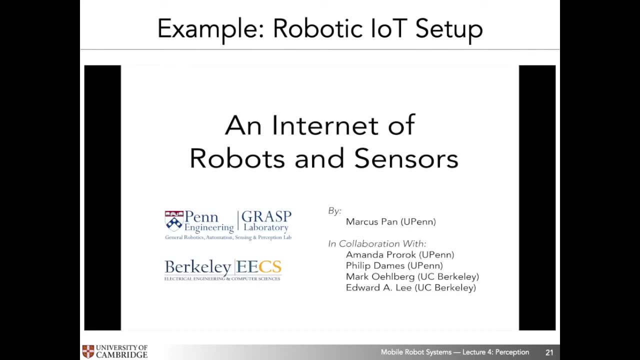 I encourage you to look up the original paper that was published in 2011,. okay, And I'm going to show you two examples of how we might actually use April Tags to do some cool things with mobile robots. So the first example I'm going to show you here: 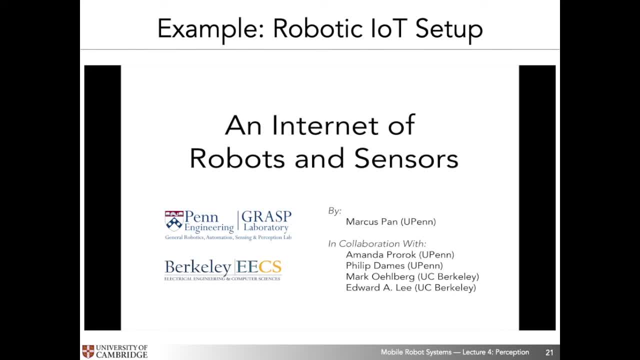 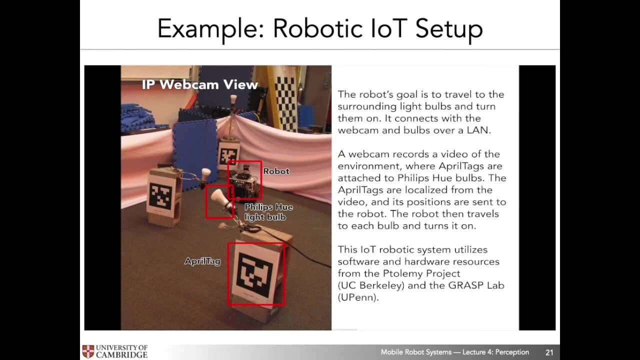 is using a combination of fiducial markers placed on static objects in combination with these objects being accessible over the internet, so over IP addresses. So let me just play this movie. So here you see a setup with a mobile robot and hue lamps that are connected to the internet. 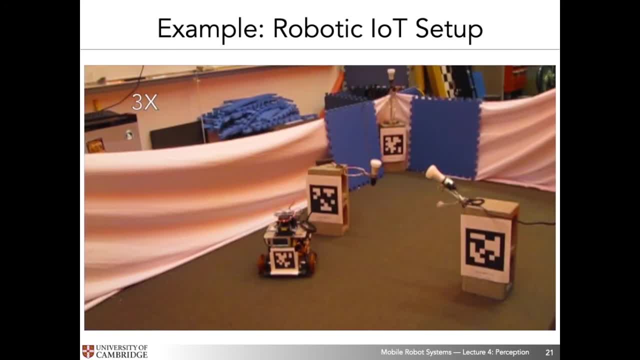 The robot can talk to the internet and can tell the network which hue lamps it's seeing, given that it detects a given April Tag, right, So it knows which hue lamp it wants to turn on once it knows which April Tag it's standing in front of. 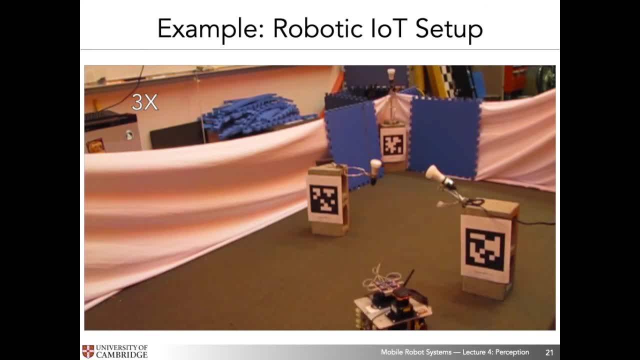 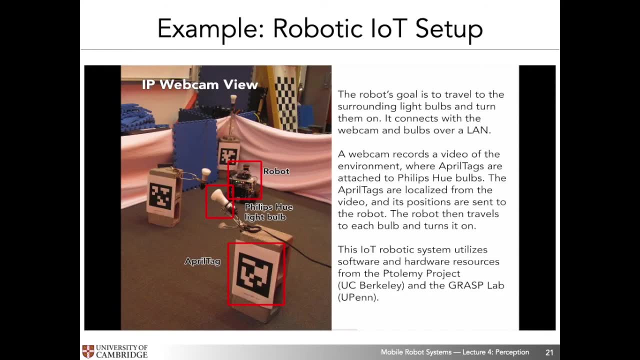 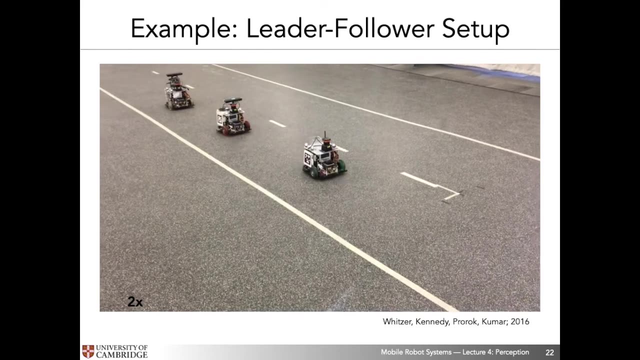 and it does that detection, given its onboard camera, And this is really cool because actually the nice thing about this is that you can connect this all up and control the robot and the access of the hue lamps over the internet. Another example that is really cool here is: 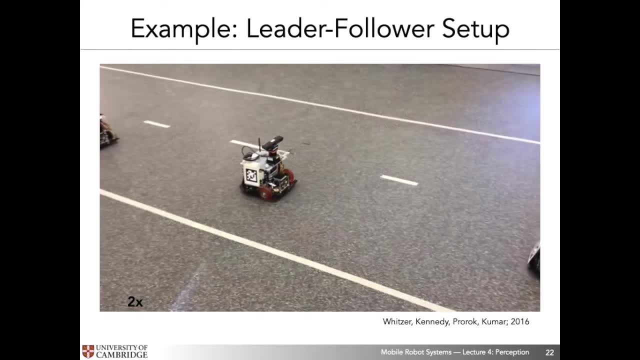 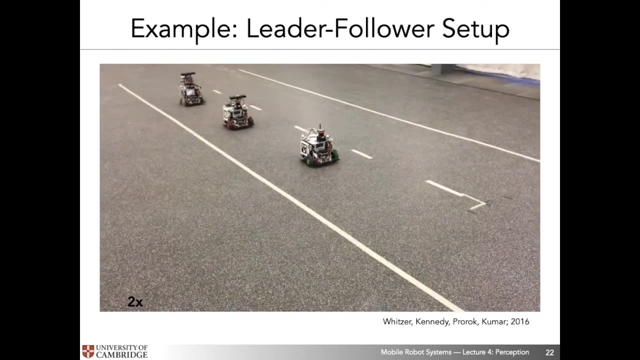 you can actually control a platoon of robots. So you can see that the two follower robots are using cameras to maintain a range as well as a bearing to the leader robot. So if the leader robot stops, the follower robots detect that they're getting too close. 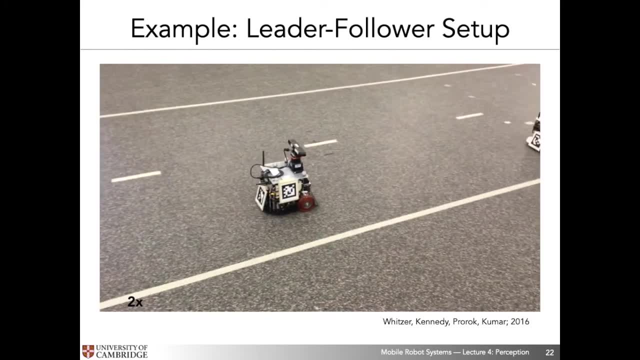 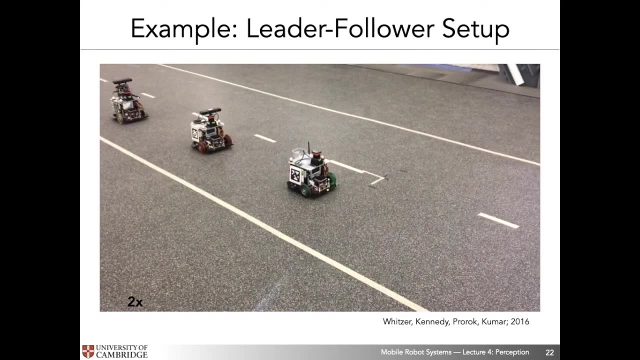 to the fiducial marker they're following and they will also stop. And as the leader robot starts turning, the follower robots will also start turning, given that they are told to maintain a certain range and bearing to the fiducial markers they're supposed to follow. right. 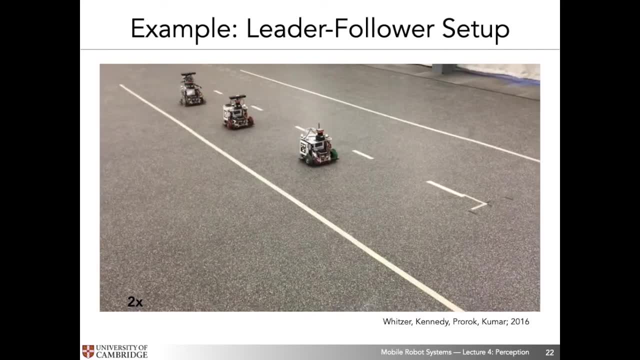 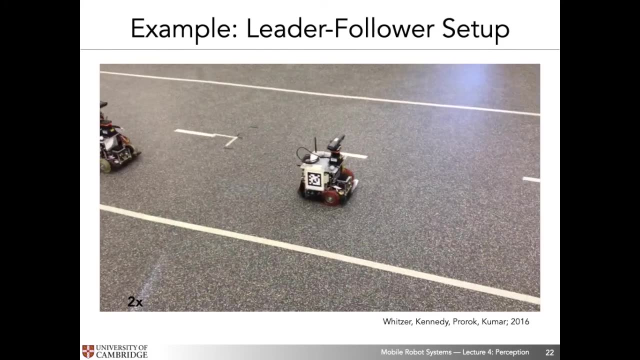 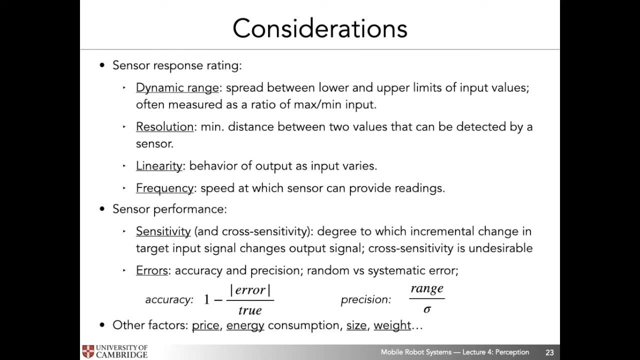 And of course you can think of more sophisticated multi-robot type formations that you can do using these April Tags as fiducial markers. So now that we've kind of looked at different types of sensors, I want to spend a few minutes talking about the considerations. 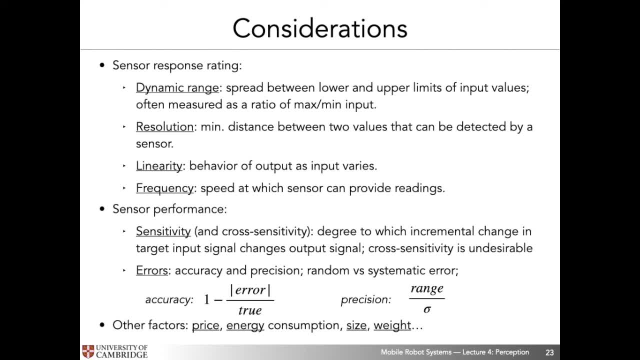 that we would need to make when we're actually choosing a sensor to integrate on a given robotic platform. So a couple of or four main components or aspects we need to consider are as follows, And the first one is dynamic range, where the dynamic range tells us what the spread is. 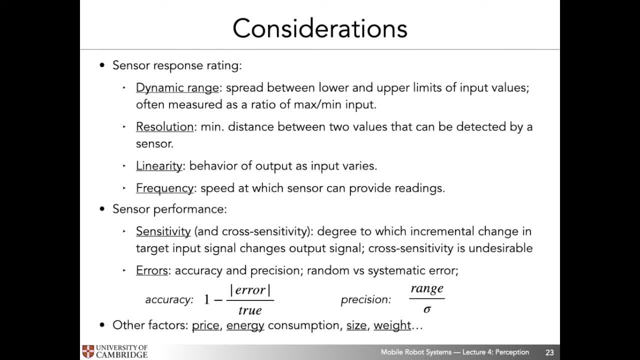 between the lower and upper limits of the input values? right, And this is important because we want to know what types of inputs we're expecting in a given environment and how those inputs relate to the task that we're trying to solve. So does the dynamic range cover the task specification right? 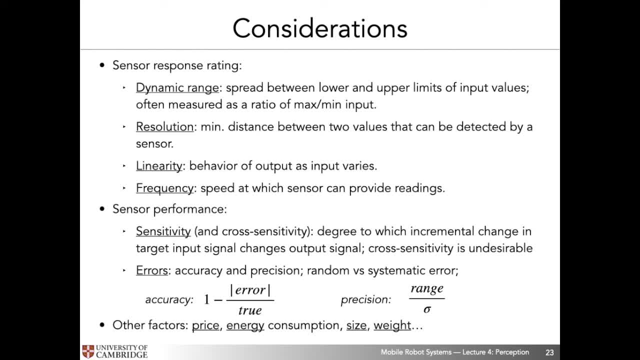 Then we have resolution. So this is equal to the minimum distance between two values that can be detected by a sensor right. So the higher the resolution, the more information we get. So we want to make sure that the information we're getting is enough to solve the task we're trying to solve. 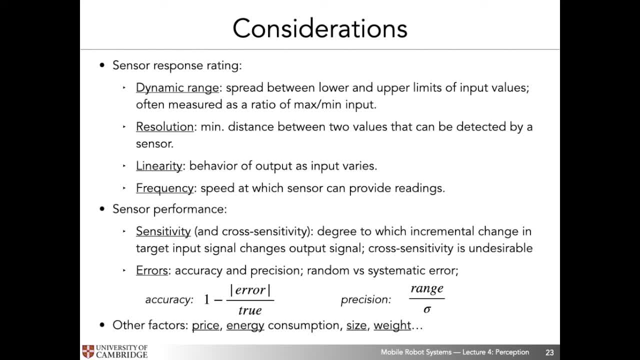 Linearity is something we may be interested in because it's practical. So does the output vary linearly or non-linearly as our input varies, And is this important with respect to the task we're trying to solve? And, of course, frequency? 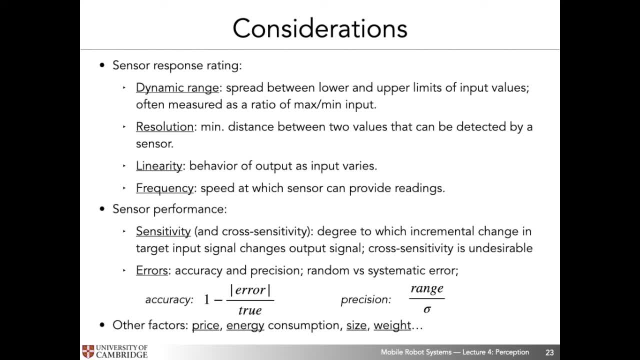 So how dynamic are we expecting our environment to be? How quickly does our robot need to react? And this is a very important question, especially if we're thinking of robots that really depend on high frequencies to maintain, say, stability or to maintain hover. 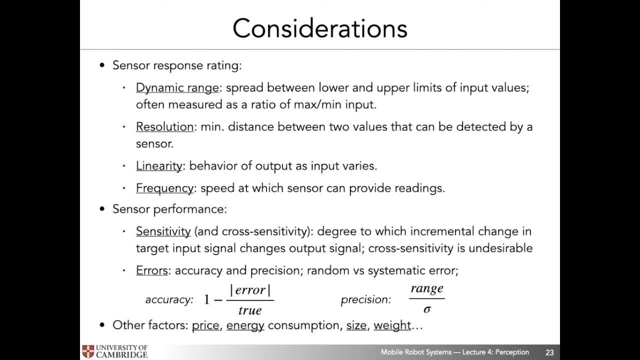 or simply maintain feasible motion right. So frequency of updates is very important for several types of robot platforms. Sensor performance also plays a role. So the first thing we need to consider is sensitivity, or cross sensitivity, which is the degree to which an incremental change 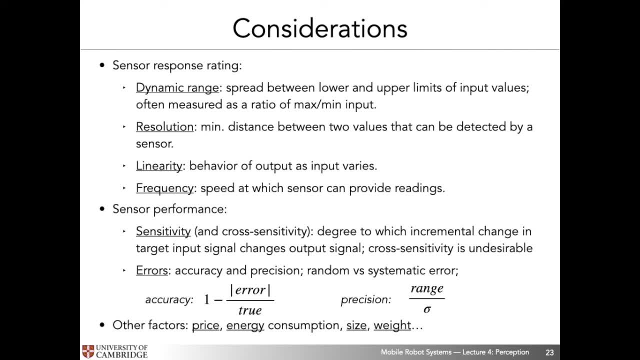 in the target input signal changes the output signal right, And so cross sensitivity is something that is undesirable. So, for example, a compass that is sensitive to a magnetic north might also be sensitive to a Ferris building right, And this is something we ideally would want. 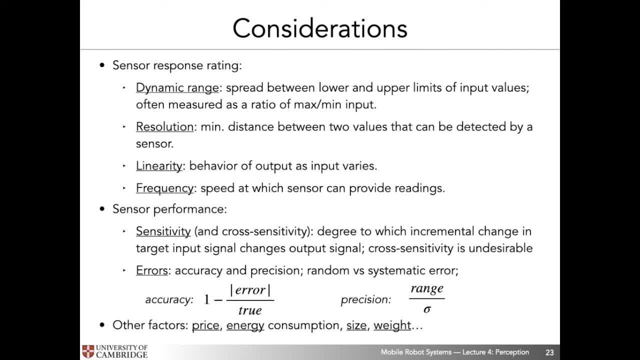 to avoid. And, finally, we want to consider what type of performance we're expecting in terms of errors. So, typically, errors are measured by either accuracy or precision, or both, where accuracy is telling us how close we are to the truth and precision is telling us how spread out we are. 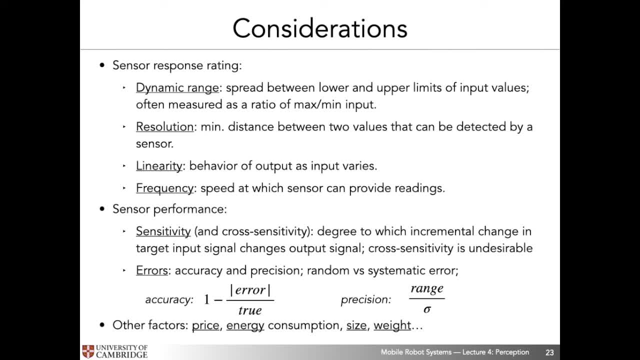 around this accuracy right, And ideally we want both high accuracy and precision. And then, finally, other factors to consider are, of course, the price, energy consumption, the size and the weight of the sensors, et cetera. okay, 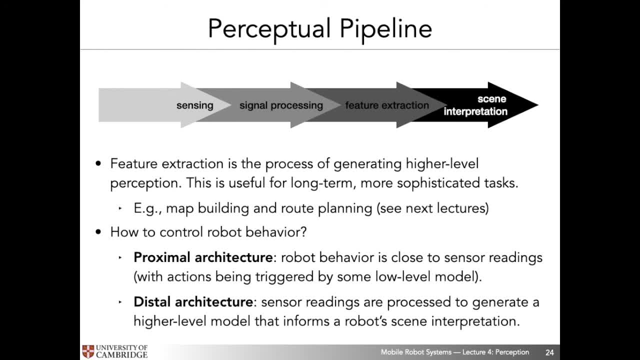 So just to summarize a little bit of what we've seen so far, we've looked at inference today by means of a relatively simple and singular sensor model, But in general in robotics we actually talk about perception as a concatenation of modules, And in this case 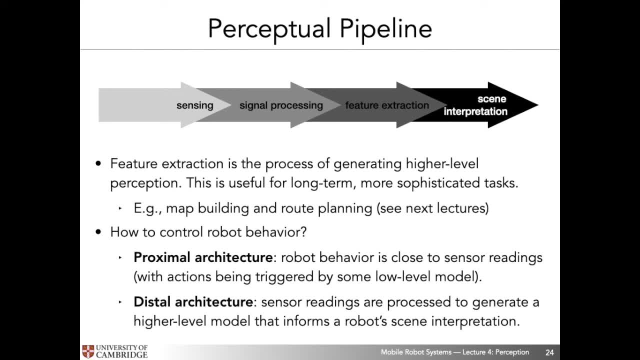 we're talking about models within a general perceptual pipeline. So sensing in general would, or perception in general would, consist of first the sensing process, Then we might be using some signal processing to process the raw signal values, Then we might feed that into a feature extraction component. 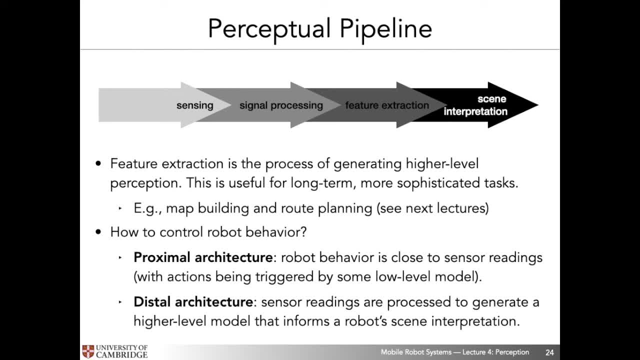 via some inference model that may or may not be similar to the models we looked at today. And, finally, we would use that output to interpret a scene or the state of the robot or the world right, And so this altogether is our perceptual pipeline. 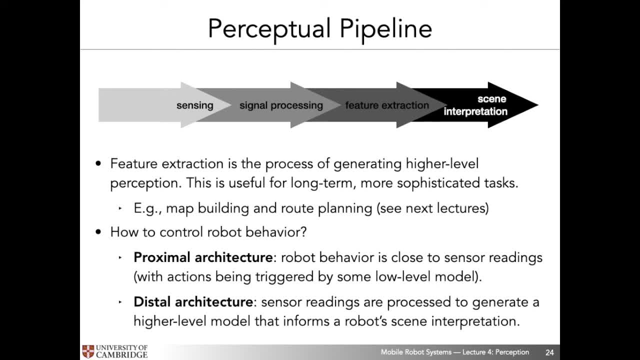 And the length or the sophistication of this pipeline tells us whether we're using a proximal architecture, whereby we'd be thinking of a very short or very simple pipeline, versus a more distal architecture, where we're looking at a long pipeline with a lot of sophisticated modules. right, 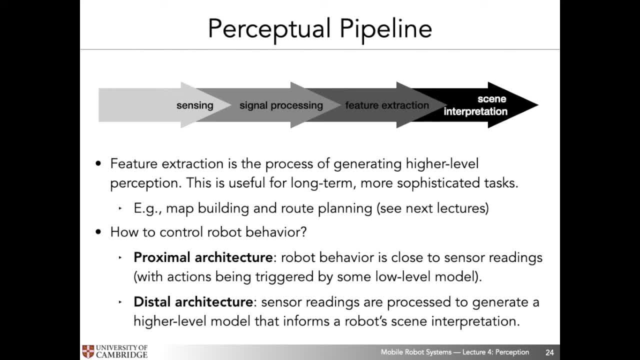 And so this then ties back to some of the very early concepts I talked about in our control architectures course, where I made the example of, for example, Breitenberg vehicles, which are clearly very proximal, And you can see now by adding all these layers of modeling. 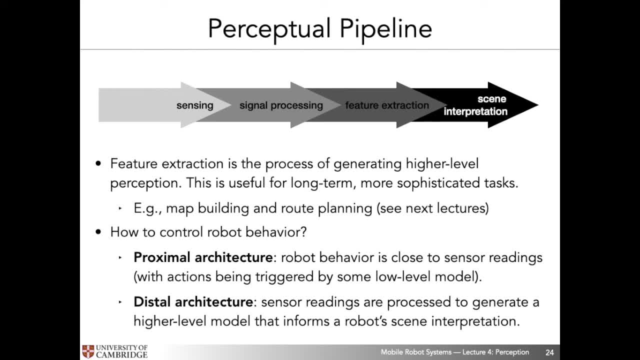 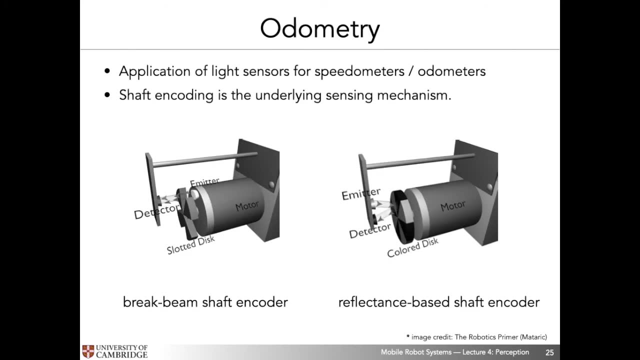 and perception and representation. we can make these architecture more distal and more sophisticated and ultimately also more powerful. So so far we've talked about extra-receptive sensing in the form of distance sensors, Now a key sensor on all mobile wheel robots. 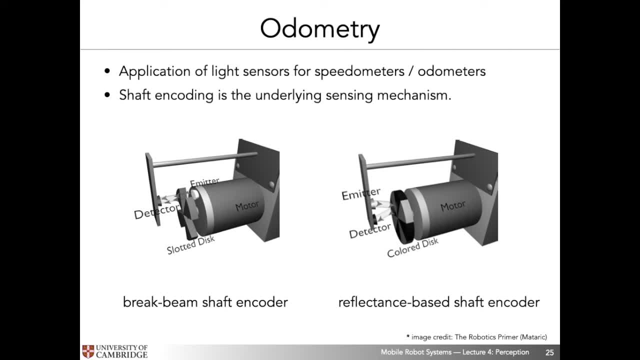 is the odometer, which allows us to measure how far a robot has moved. So odometers are based on this concept of shaft encoders that allows to measure the angular rotation of a shaft or an axle. And how do they do this? Well, it's a simple application of light. 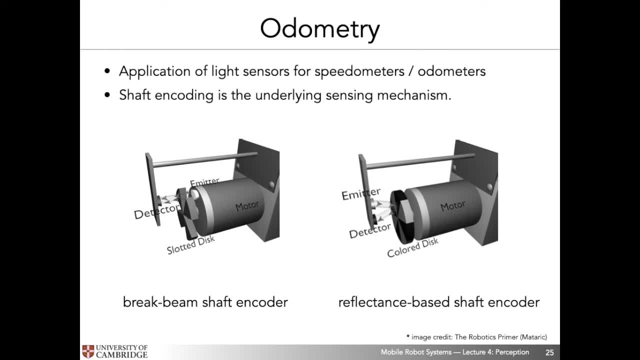 and based on the combination of that, with two different options or two different ideas. So the first idea is given to us by the brake beam shaft encoder, which basically uses a slotted disk that breaks the beam that is being emitted by the emitter that moves around with the motor. 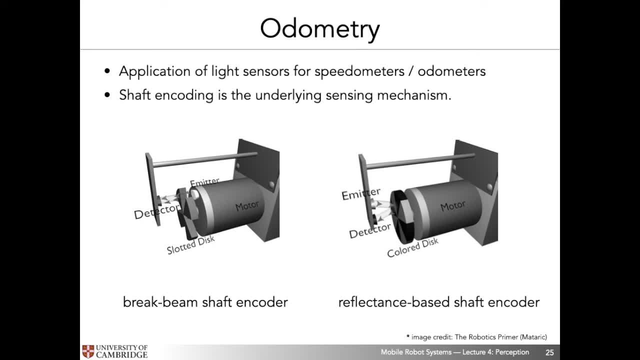 And the second idea is our reflectance-based shaft encoder. that is basically based on the idea of a colored disk that affects the sensor reading. So you can see here how we have an emitter emitting the light in the detector, detecting the returned reflected light intensity. 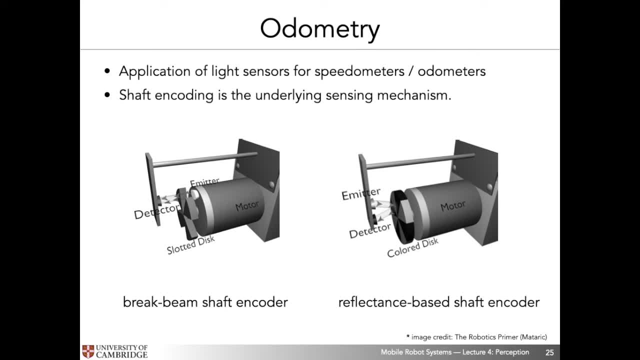 based on the color that is moving around, so that color disk that is moving around attached to the motor. So these are the two options that we have for light-based shaft encoding And in both cases, what you're doing is you're measuring the rotation of the wheel. 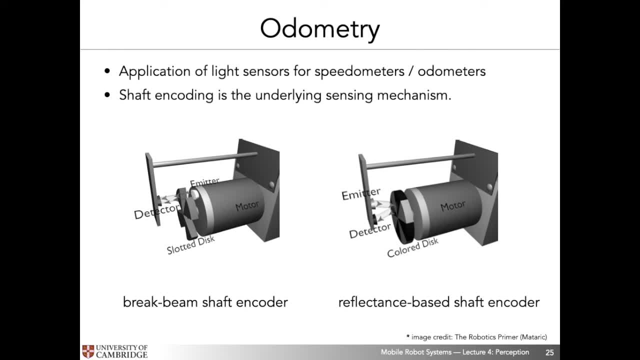 which is very practical if you want to measure how far your robots are moving, And so these kinds of odometers, or also speedometers, use ideas as such to determine how far they're traveling or at which speeds. Now one more thing that you can do. 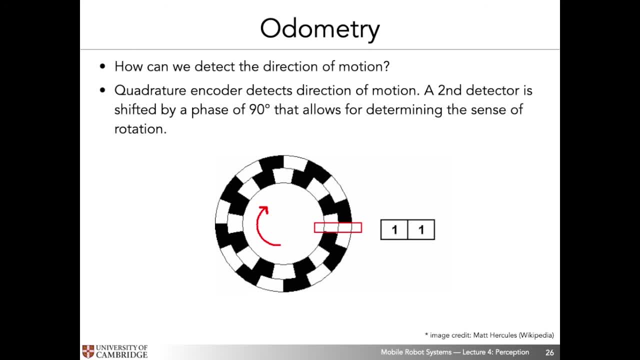 with odometers is you can also use the shaft encoders to measure the direction of motion. So how would we do this? So the quadrature encoder here is able to detect the direction of motion where a second detector is shifted by a phase of 90 degrees. 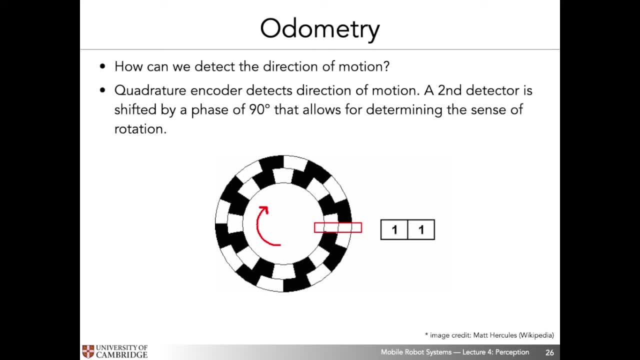 that allows for backing out what the sense is of the rotation. So if I play this GIF here, you can see how the transition of the encodings differ as you move in clockwise versus counterclockwise directions. right, So if you're working in clockwise, 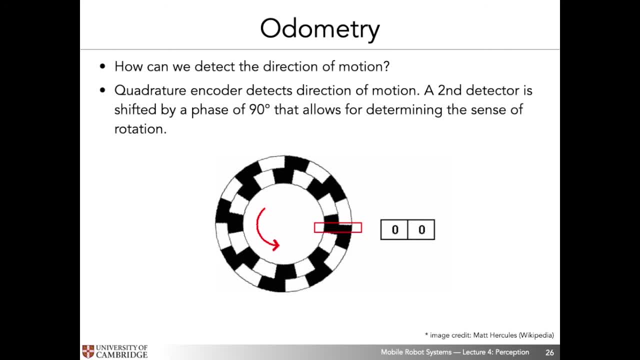 you would detect the transitions of 11 to 01 to 00 to 10, right If we encode white with 1 and 0 with black, And in the case of counterclockwise, the transitions you'd be encountering here are 11, 10,, 00, and 01, right. 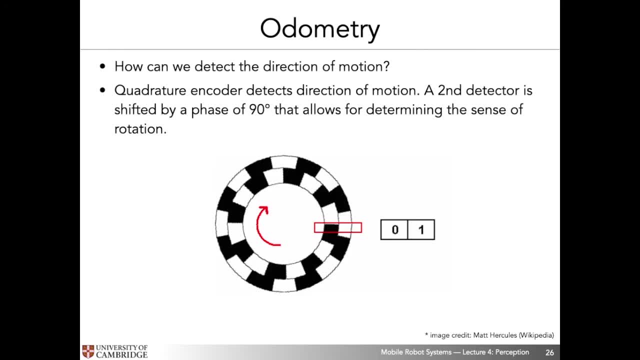 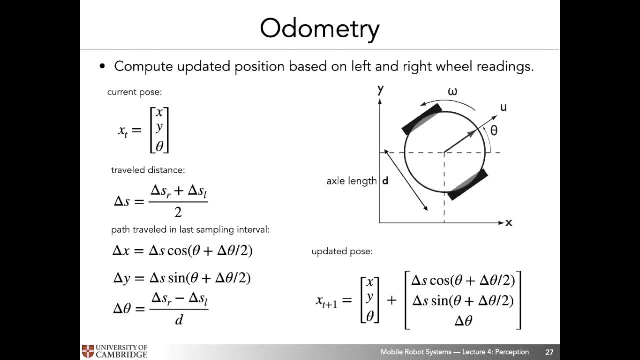 So the transitions are different and this is how you would be able to detect the direction of motion. So now the question is: how do we use these readings for the purpose of odometry? So what we want to do in odometry is we want to compute. 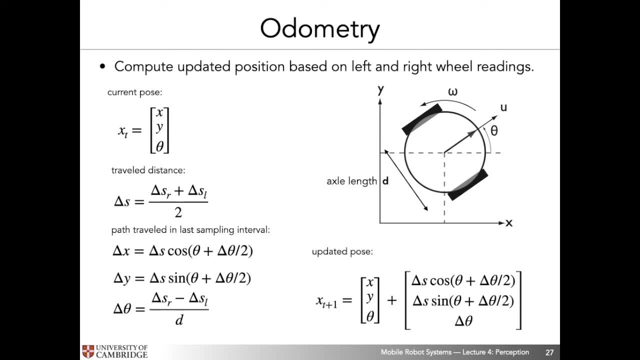 the robot's updated position based on these left and right wheel readings. Now, first we're going to assume that we have knowledge of the robot's current state or its current pose, given by x, y and theta. so x- y, position and orientation, theta: 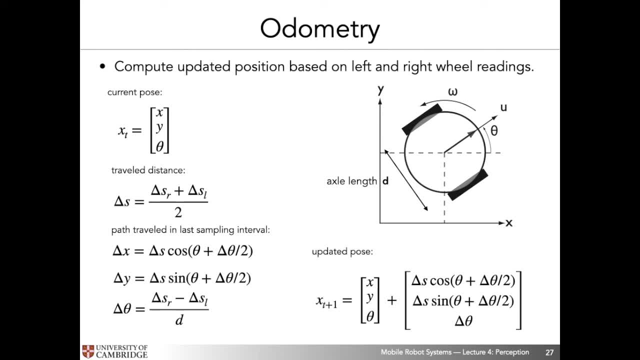 in some given coordinate frame And our odometers are going to give us the readings delta s for the left and right wheels right. So the travel distance will then be equivalent to our delta s, which is given to us by this equation here on the panel. 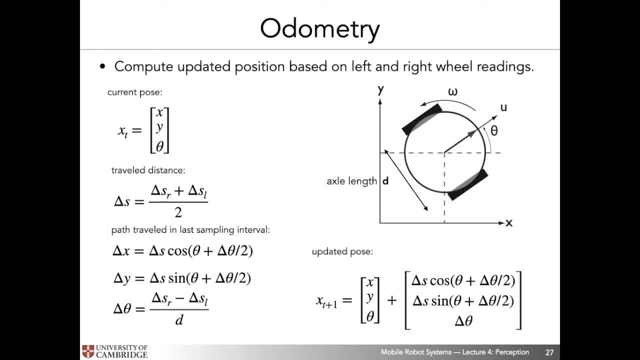 And so, finally, we can use the knowledge of the robot's previous pose and the updated travel distance equation to compute delta x, delta y and delta theta in our given coordinate frame, where our goal is to update the robot's pose in this given frame. 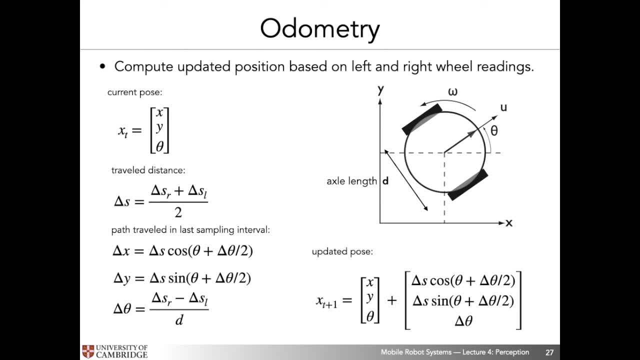 So now, looking at the equation on the right-hand side, we simply have x at time. t plus 1, assuming we know what our sampling frequency is- is simply equal to our robot's pose at the prior time step, plus this travel distance for x, y. 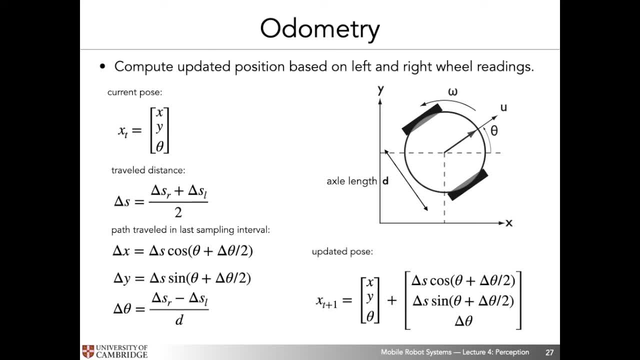 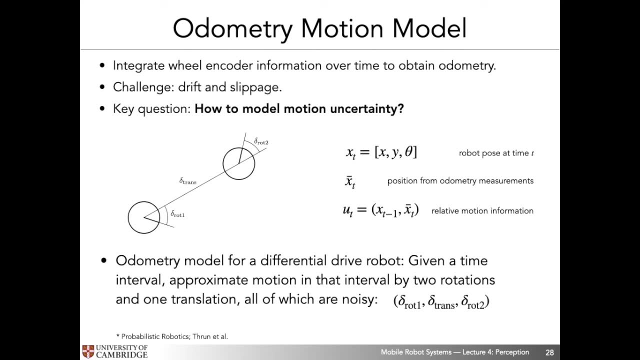 and our delta, theta for our orientation right. So since odometers are also sensors, these odometers will also require sensor models. Since odometers are no different, they are also susceptible to noise, and we need to have a way of modeling this uncertainty. 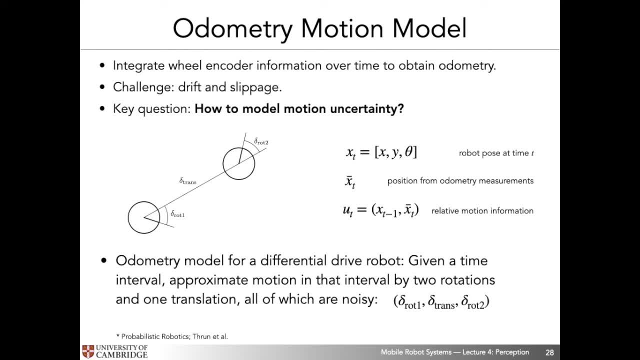 that is given to us through the noise that they are sensitive to, And there are, of course, various ways again of doing this, and the method that I'm going to be introducing to you today is based on the methodology that is described in Trone's book. 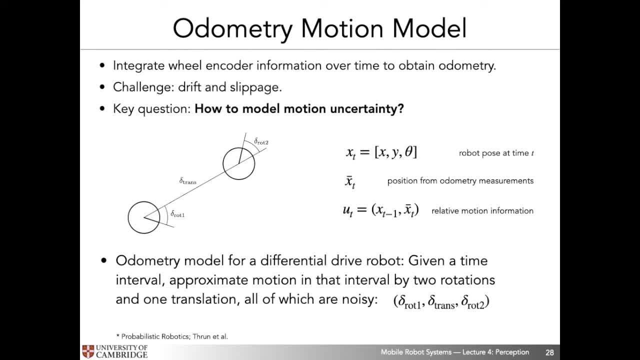 and I do invite you to have a deeper look and deep dive into that method in your free time. So what we're going to do is we're going to look at how integrating wheel encoder information over time gives us odometry and how to interpret that odometry measurement. 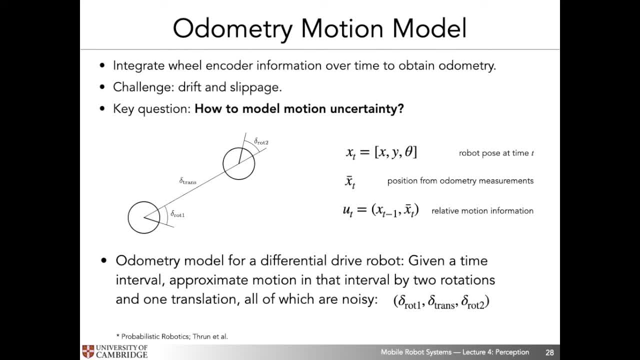 when we know that there is uncertainty. So uncertainty is, in this particular case, when we have wheel slippage, or wheel motion is most often due to drift in the actuation mechanism or slippage between the wheel and the surface that it is moving on. 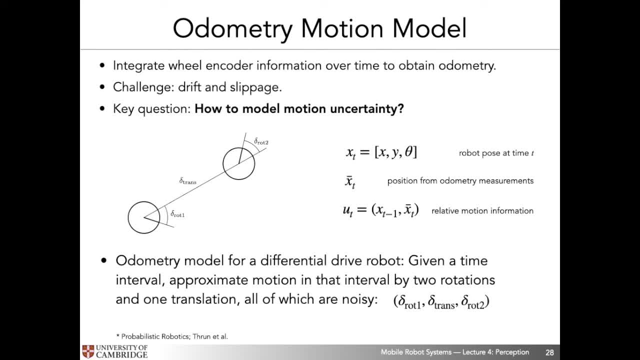 Now, how are we going to model that uncertainty? Well, the first thing that we need to do is to simplify the motion of, or the way we're thinking about it, or the way we're thinking about how a robot moves between point A and point B. 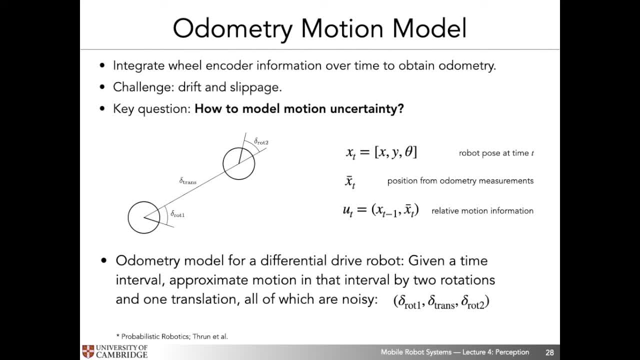 in a given time interval, And the way that Trone introduces this is by assuming that the motion in a given time interval can be represented by two rotations and one translation. So if we look at that image in the center of this panel, we have robot pose at time A and time B. 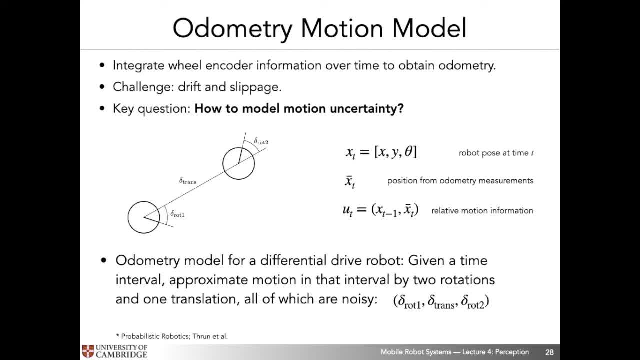 for example, given by x, y, z, And we then transform the translation and rotation into d-rot1,, d-rot2, and d-trans. So you see, with these three components we can transform any robot translation rotation from one point to another. 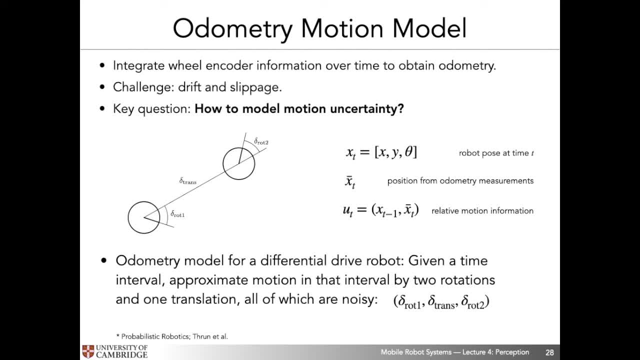 into these three different components, And the notation that we're going to use here is to say that x sub t is a robot's pose at time, t, x bar is its position, that is inferred through odometry measurements, and u of t is the motion information. 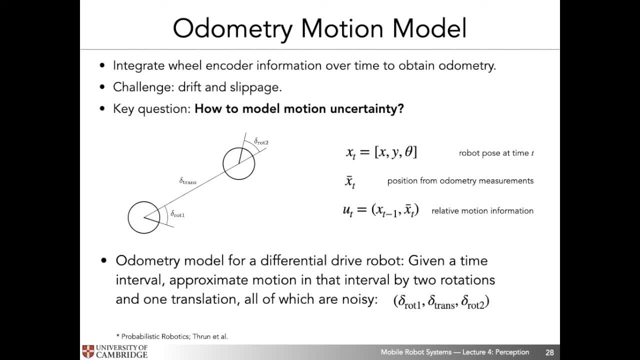 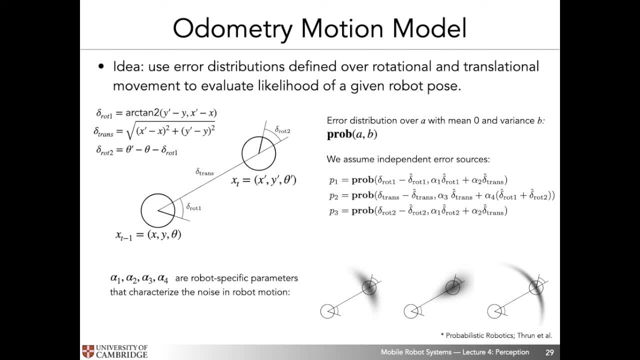 relative to our prior pose x at t minus 1.. So the idea that we're going to leverage in order to model the motion uncertainty or the odometry uncertainty is to use error distributions that are defined over these three components that we used before to describe the change. 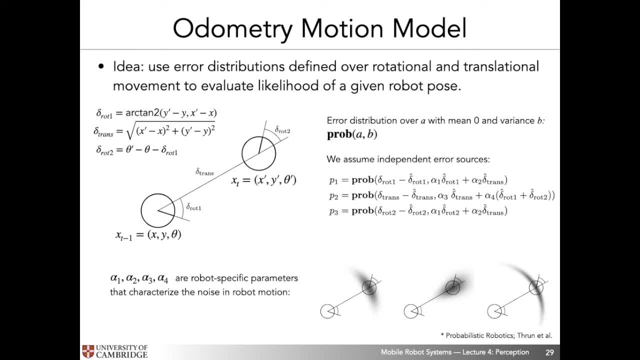 in the robot's state. So we're going to define these distributions over the two rotational motion components and the translational motion component And then we're going to use those three models to evaluate the likelihood of a given robot pose that we're trying to. 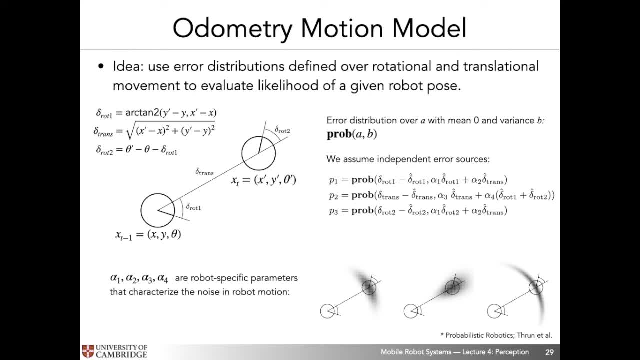 understand whether or not the robot is likely to be there or not. So the first thing we do is we describe d-rot1, d-rot2, and d-trans through these three equations that we can derive based on first principle's geometry. 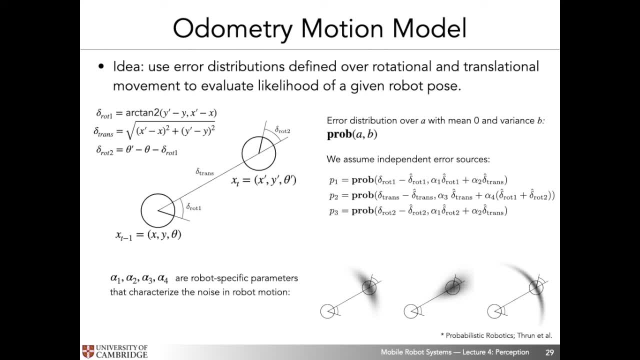 And we then say that, well, now we have descriptions of these three components. We're now going to define three error distributions, each of which will be a normal that will allow us to model how the robot's uncertainty changes as a function of certain motion parameters. 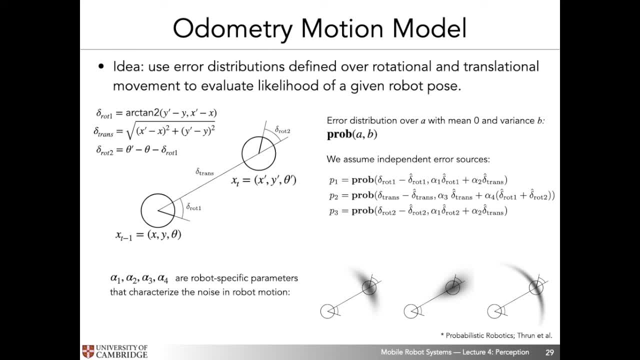 And these motion parameters, alpha1 to alpha4, are described in more detail in Tron's book and I invite you to have a look at them because they have different effects On the way that we represent how motion uncertainty propagates throughout time. Now, in terms of notation, 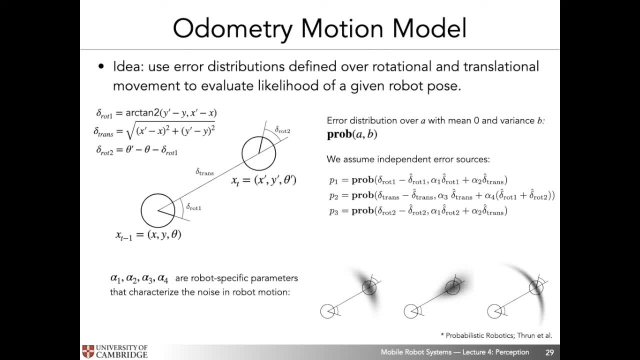 I just want to spend another second on that. what we'll be assuming here is that d-rot, for example, without the hat, represents our odometry measurements to a new point. So d-rot tells us how we've rotated from a prior point to the new point, based on 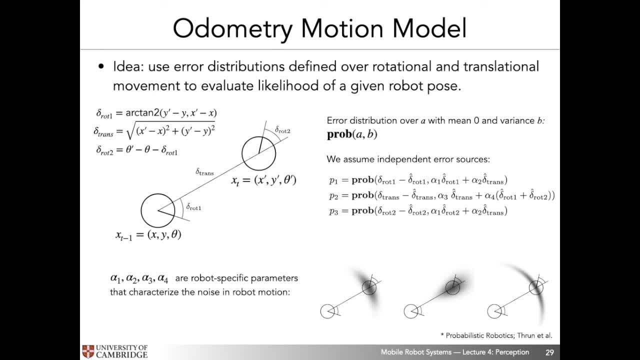 what our odometer is telling us, And d-rot hat is the quantity that tells us where the robot has rotated to with respect to the point that we now want to evaluate. So those are not the same things, So d-rot hat is. 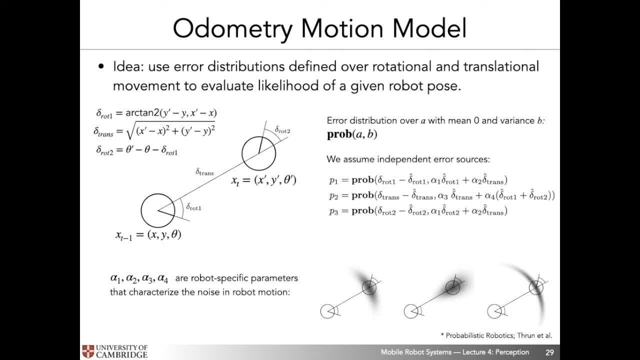 from a given point rotated to a new point, and that new point is the one we want to evaluate its likelihood. So that new point is not given to us by the odometry measurements. it's given to us by a certain position in the map we want to evaluate. 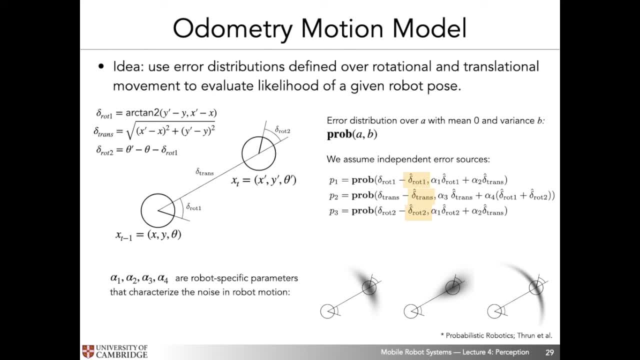 the likelihood of, And I also just want to point out that the alphas here that we use in these probability distributions, so these gaussians can be tuned to give us the noise distributions, for example, as illustrated in this sketch. So by tuning the alphas, 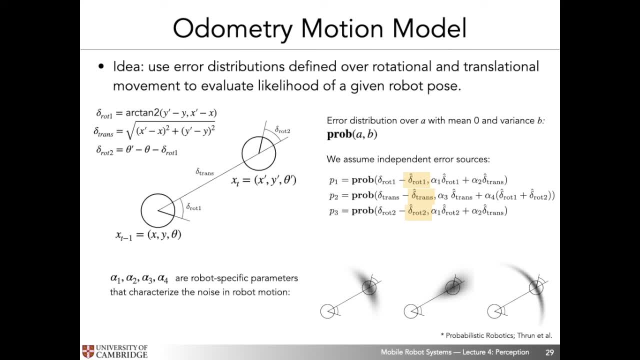 we get different types of uncertainty models, for example, more in the radial axis or more in the longitudinal axis, depending, of course, on the kinds of uncertainties we have observed in our measurement campaign. So, as any other sensor, odometers as well would need to be calibrated. 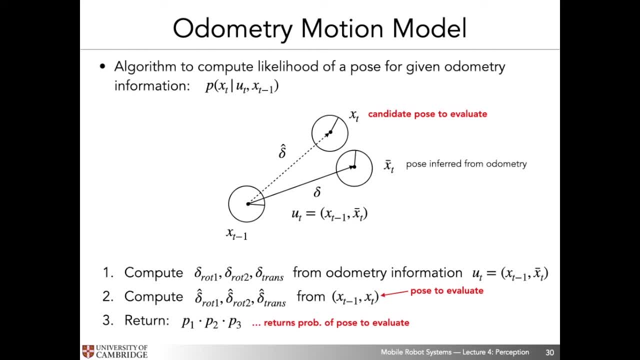 So in the next course, which will focus on localization, we will be making heavy use of this equation that is written on the top of this slide, which evaluates the probability of a candidate pose x at a given time. t, given that we know the motion that the robot exerted, so u 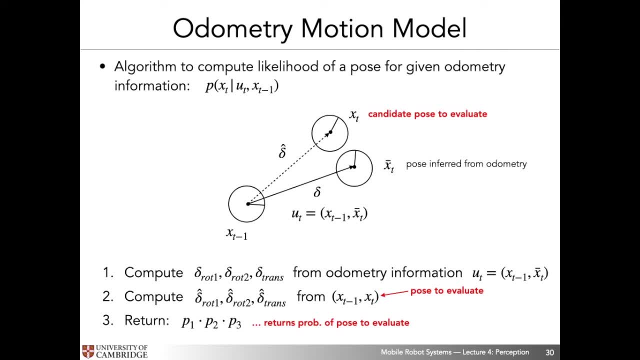 and that we know where it came from at the previous time step. so x. So what I want to do now is go through how we actually compute this probability. So recall first of all that we assume we know where the robot is coming from at the previous time step. 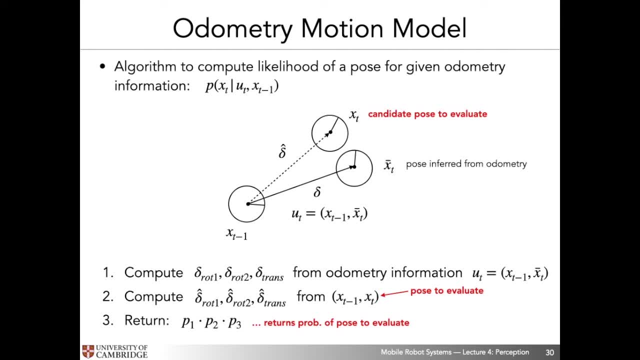 and that odometry is going to tell us how our robot moved by the quantity u sub t, and hence we will assume that we can compute the quantity x bar, which is the new pose inferred from odometry. but what we want to do now is we want to compute a distribution. 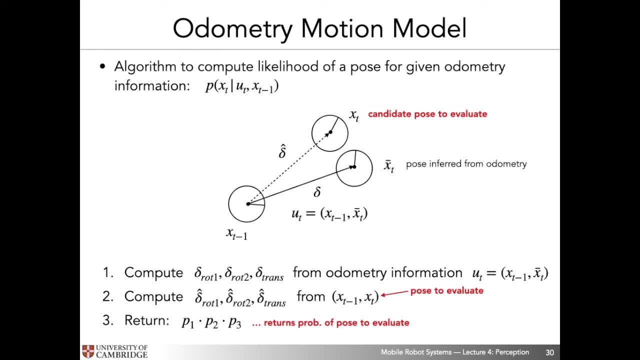 over our candidate pose x of t, so that we can essentially compute the likelihood of any given pose that we want to evaluate. So let's go through the three steps that allow us to do this. So the first step basically consists of computing our delta rod 1. 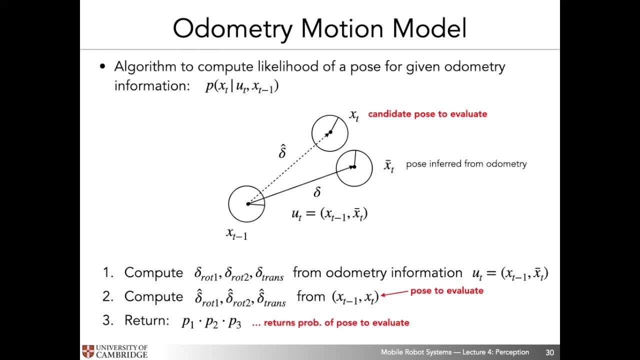 delta rod 2 and delta trans, as given in the previous slide from our odometry information u sub t. so this is all we need in order to compute those delta values. The next thing we do is we compute the delta hats where, in this function, the 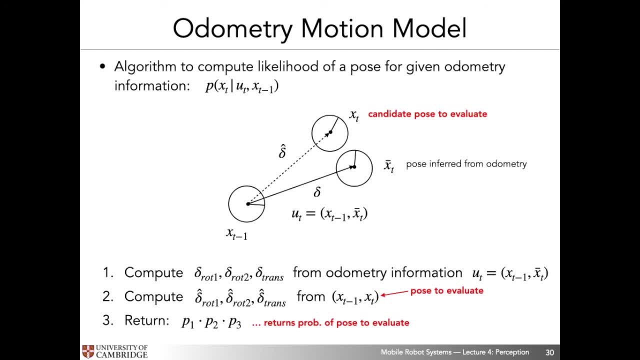 equations are simply a function of that new pose, that candidate pose that we want to evaluate, and otherwise equations are similar. And in the third step we compute those three probability values as given in the prior slide, and we then compose them to return a joint probability. 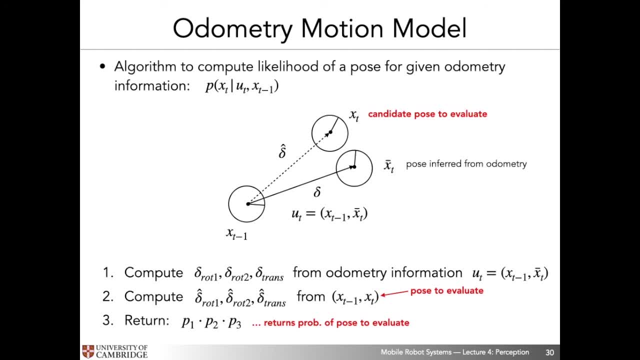 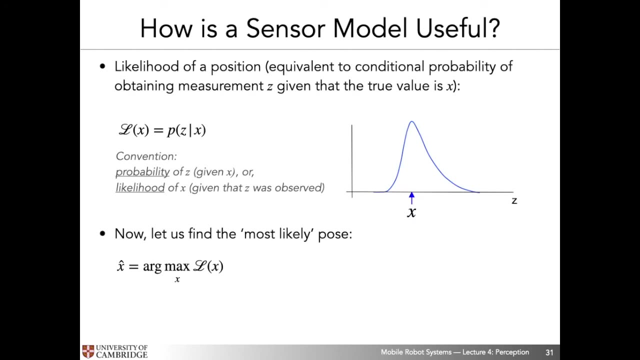 of the pose that we're considering to evaluate. so x, sub t. So those are the three steps that we would go about to compute the likelihood of a candidate pose. So now, finally, I know we've gone through a lot of material, but as a small interlude, 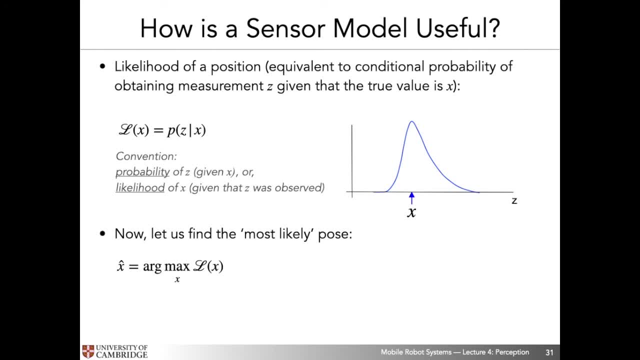 to the next lecture. I would like to give you a mathematical intuition about how sensor models are employed when we actually have information from several sensors. So this idea of sensor fusion is extremely popular and common in robotics because more often than not, we're using more than one sensor. 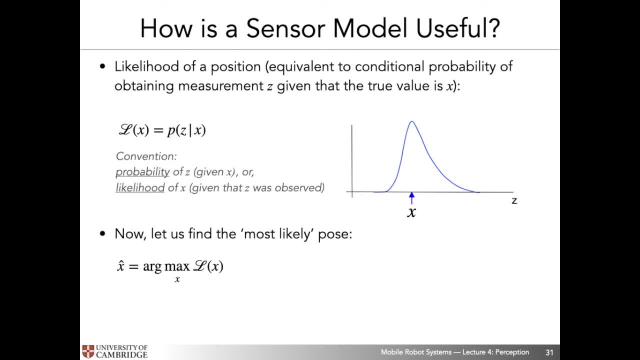 and how to combine the information coming from several sensor streams in a probabilistically or formally sound way is really key to the perception problem, And so what we're going to do today is we're going to look through how we actually compute the likelihood of a given position. 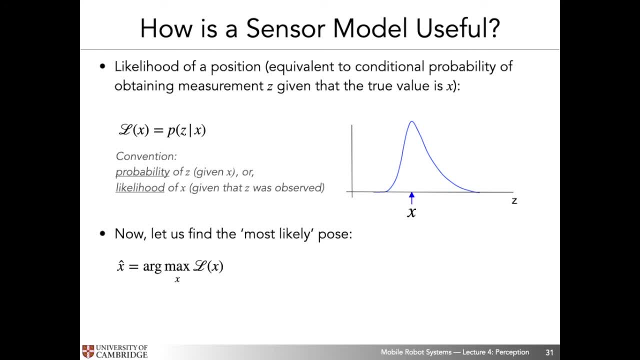 So the convention is that we say that we have the likelihood of x, which is equal to p, of z, given x, which is equivalent to saying that we have the probability of a given measurement, z, given that we know the position x, or we assume we know the position x that it was measured at. 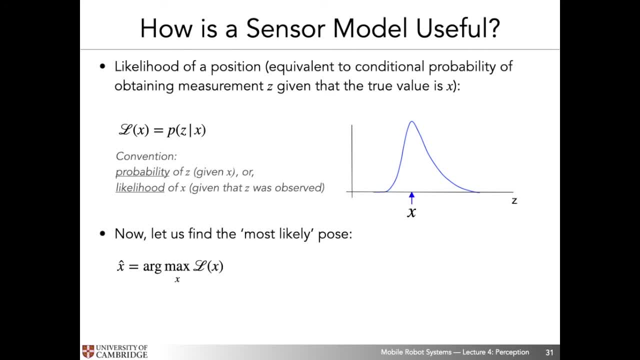 or we have the likelihood of a given position or pose x, given that we know that z was observed. So these two things are equivalent. So L is the probability of z given x or the likelihood of a pose x, given that z was observed. So these are two ways of reading. 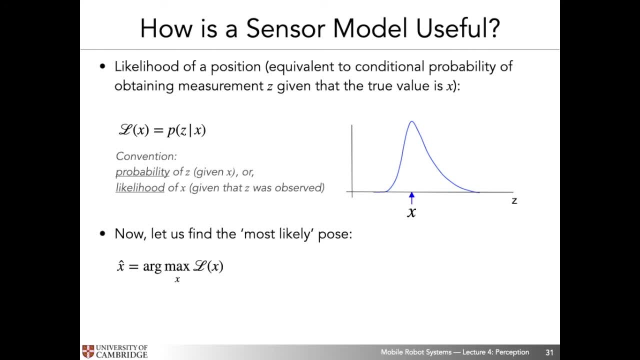 this equation. Now what we want to do is we would like to find out what the most likely pose is, given that we made a certain sensor observation, And the way we're going to do that is we're going to maximize this likelihood over all candidate pose values x. 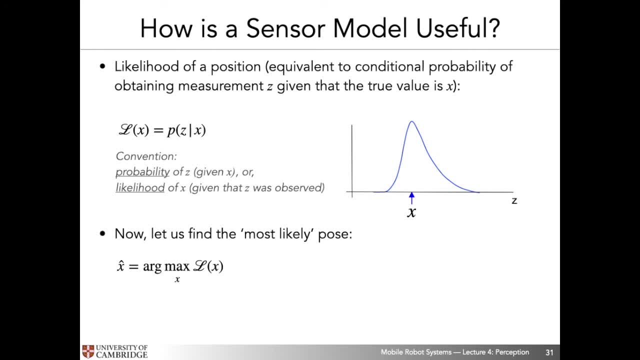 And that will give us our most likely pose And, in turn, will tell us where our robot is located. So this is really the core problem underlying the localization problem in robotics. So what we're going to do is we're going to use a method called maximum likelihood estimation. 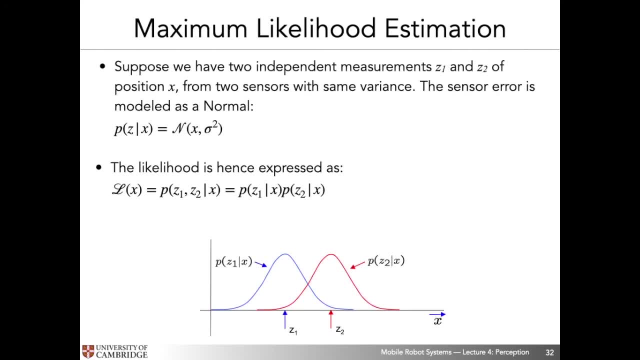 in order to do this. So, first of all, what we're going to do is we're going to assume that we have observed two sensor measurements, z1 and z2, that were both taken in position x from two sensors that have the same variance. But we do. 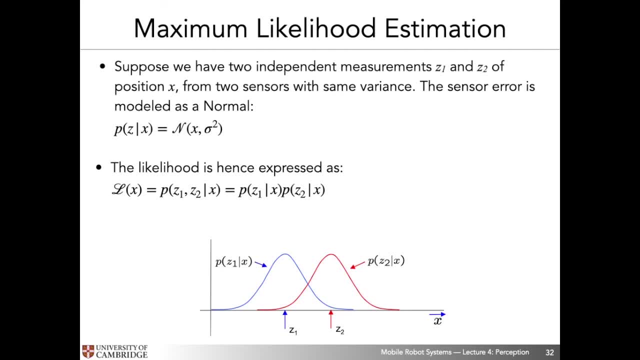 however, assume that these two sensor readings are independent, otherwise, And we're going to model the sensor error as a normal, so a Gaussian. Now, schematically, we might think of drawing this as shown in the panel here, where the blue curve corresponds to the sensor model of: 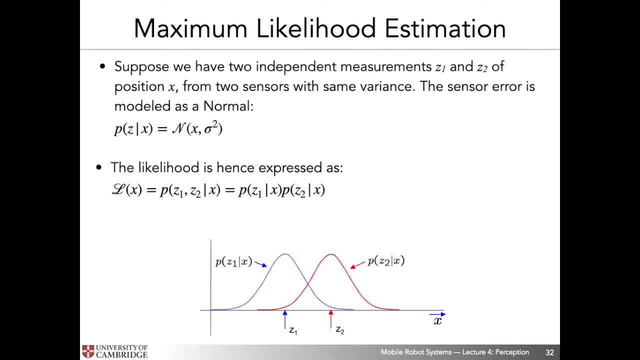 our first sensor, and the red curve corresponds to the sensor model of our second sensor, And of course they're centered at this point here around the sensor readings that were observed by the sensors. The likelihood then is expressed as p, given x, which is equivalent to. 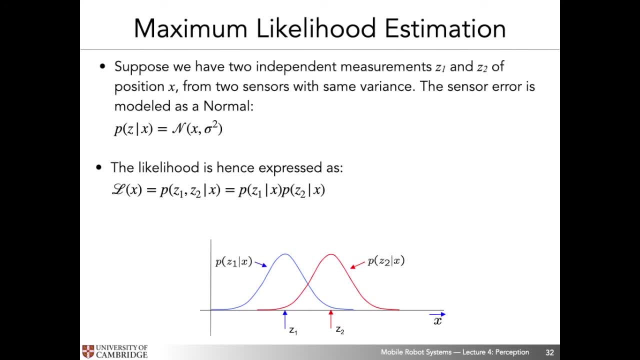 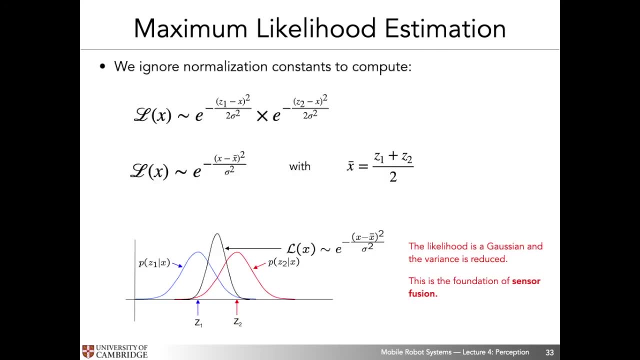 these two probability density functions multiplied by each other, because we know that these two sensor readings are independent, or we assume they are. So now, given that we are assuming Gaussian distributions over x, with mean z1 and z2 and the same variance, we can rewrite these equations. 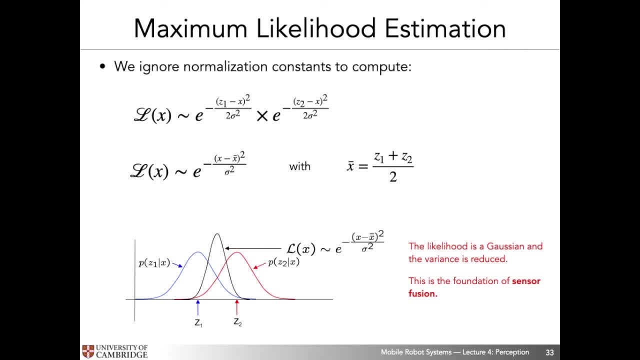 as written in the first line. This is simply the two probability density functions multiplied with each other, And we can simplify them to give us what is written in the second line in this panel, And what you can see here is that our x bar is a new mean. 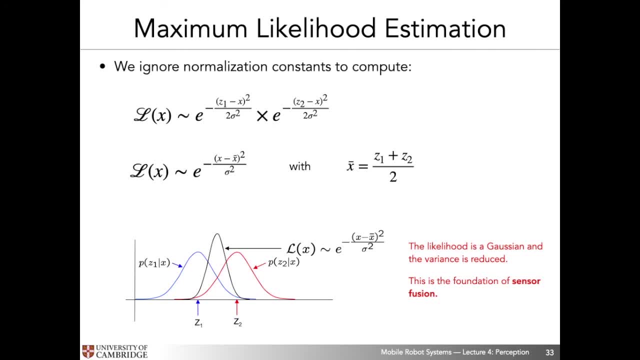 and we can see from the formula that it lies in the middle of our two former means And the new variance here, described by this new Gaussian that we obtained. this simplified Gaussian is equivalent to the half of the original variances of the original sensor models. 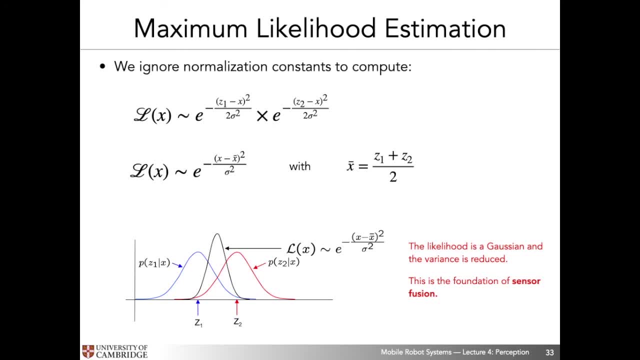 that we had given to our template model. So let me just summarize what we did here by simply simplifying the equation for the likelihood. I had two sensor measurements, both coming from sensors with the same variance, and I now have a new distribution that describes the likelihood of oppose x. 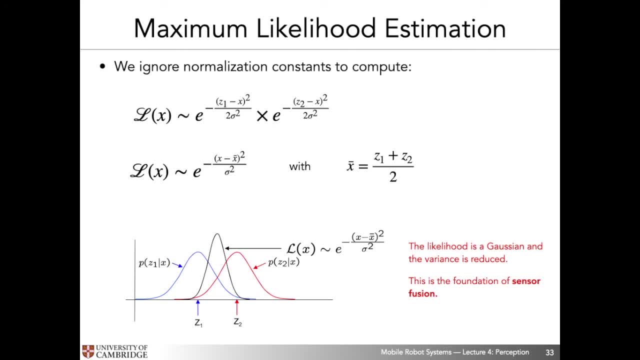 which has a narrower variance, and its mean is a compromise of the observed means that we originally had. So this idea here is really the core of sensor fusion. So we're reducing uncertainty and we're compromising between sensor measurements, And this is what the math has told us that happened. 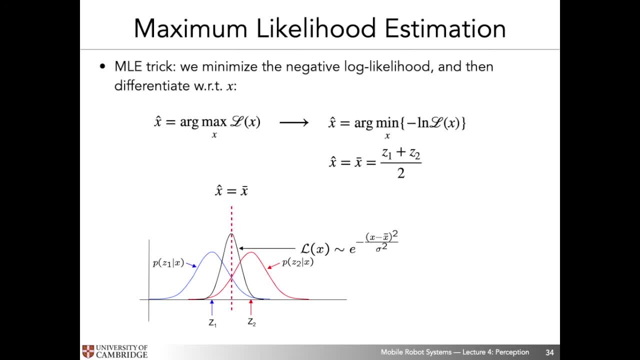 So we're not quite done yet. We have one more step to do, which is we would like to now compute our best guess for where the robot truly is positioned, given that we made these two sensor measurements. And so what we're going to do is we're going to take the argmax. 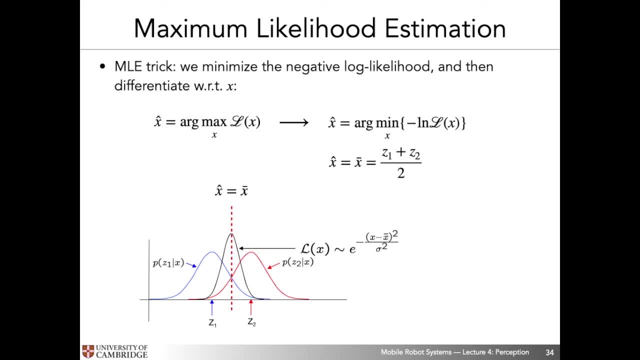 over this likelihood for all given positions over x, And for convenience, we're going to argument the negative log likelihood because it is simply easier to compute. but this is strictly equivalent, And so by computing the mean over the curve that we saw in the previous 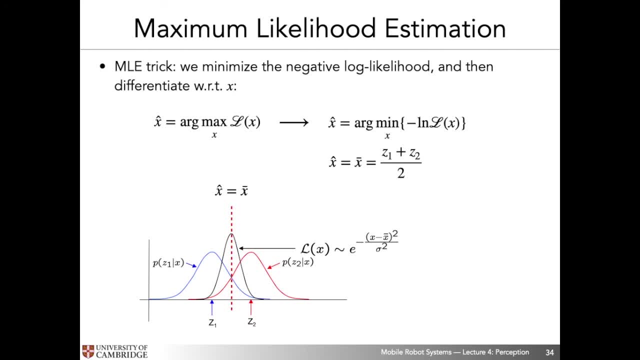 slide, we now get this new equation which tells us that x hat equals x bar equals the average of x over z1 and z2.. Which simply means that the most likely pose for the robot indeed lies in between the two sensor measurements that were read from. 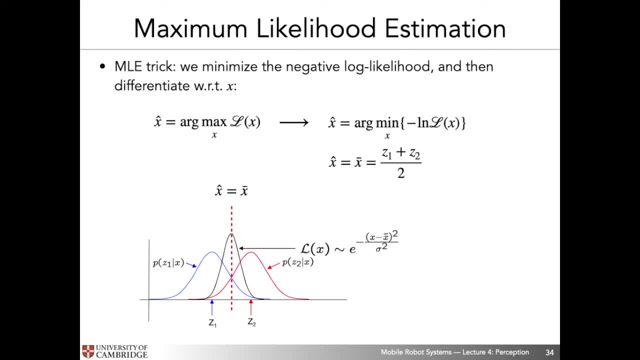 these sensors. So now we have our maximum likelihood estimate for the robot's position. And just a side note, we can do a similar computation when the variances of the two sensors are not modeled by the same variance. So what I showed you in these last two or three slides is 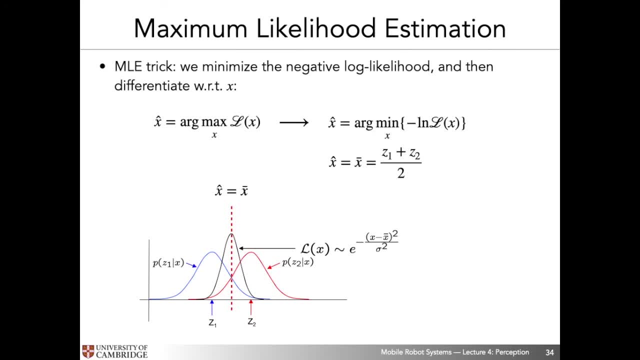 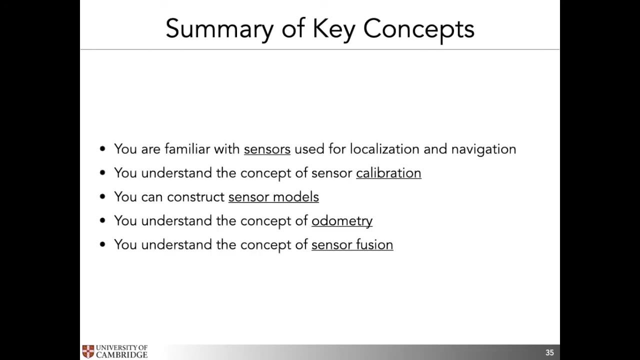 how we can actually use sensors models and how we can employ them to combine independent sensor measurements to give us estimates of where our robots are actually positioned. So, with this, this now concludes the content of today's course, and I'd just like to finish by summarizing.